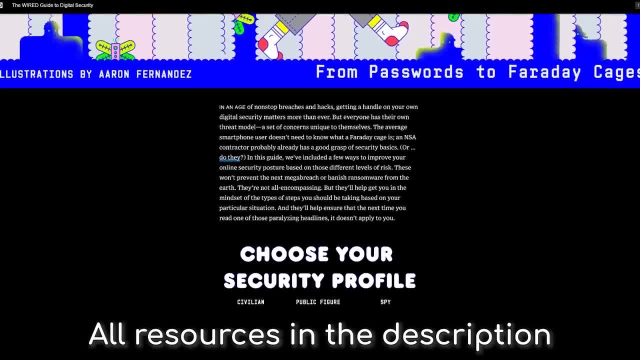 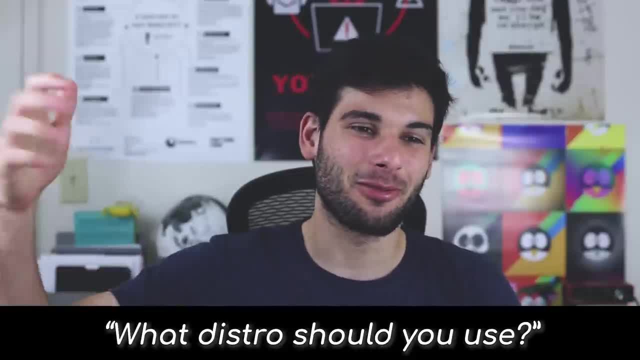 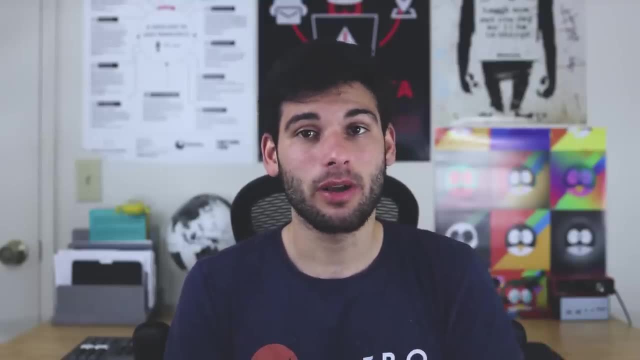 Before getting into our glorious three zones, let's address the golden question: What distro should you use? And everyone should get their swords and weapons out for this. There is no correct answer here. This is ultimately your choice and almost every distro. 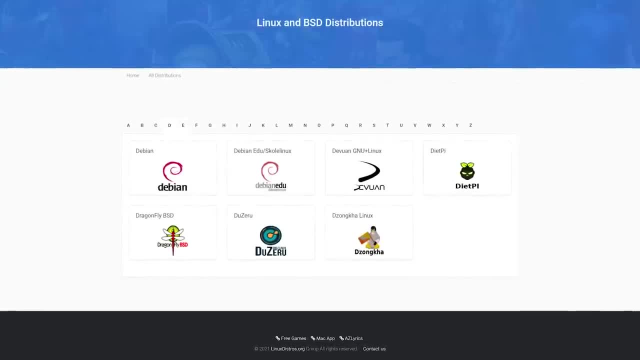 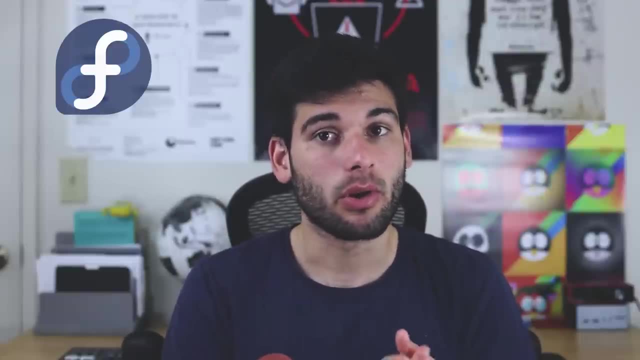 even Ubuntu is leagues ahead of things like Windows. for your privacy, Do your own research and pick what helps you the most. Our three recommendations to look into are Fedora, Fortnite and Ubuntu. If you're a fan of Fortnite, then you should definitely check out Ubuntu. 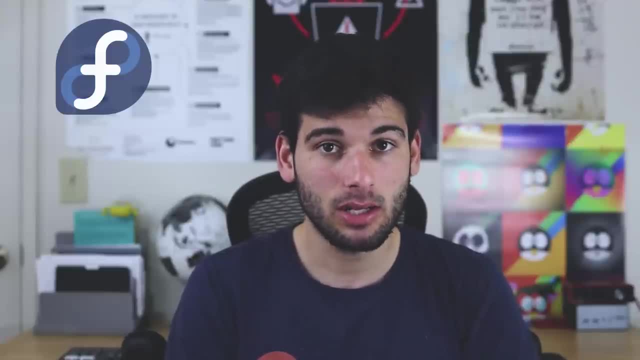 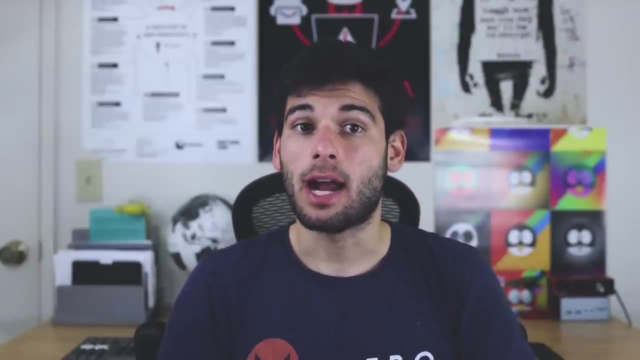 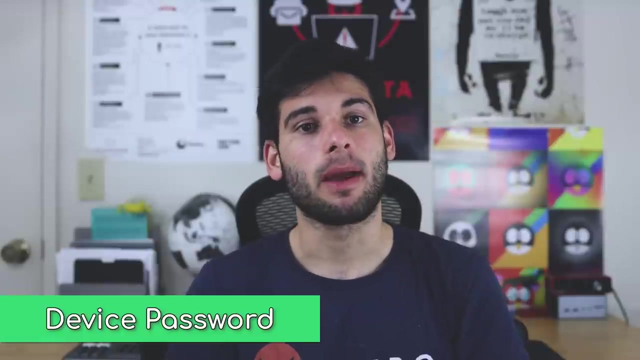 Overall, simple, easy to use distro with overall decent security. Debian and Arch For most people. we push them to Fedora, but again, this is entirely your choice. After you've chosen a distro, let's go ahead and start the zones. Your device's login password is your first form of protection. 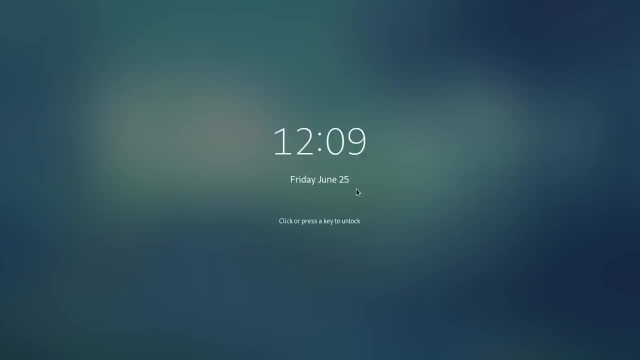 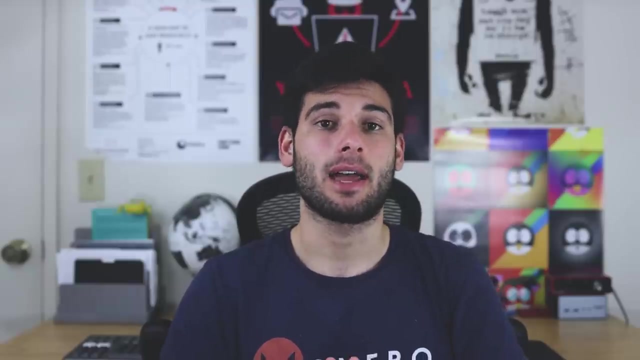 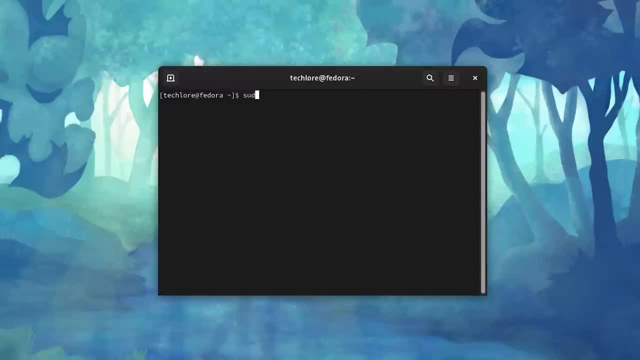 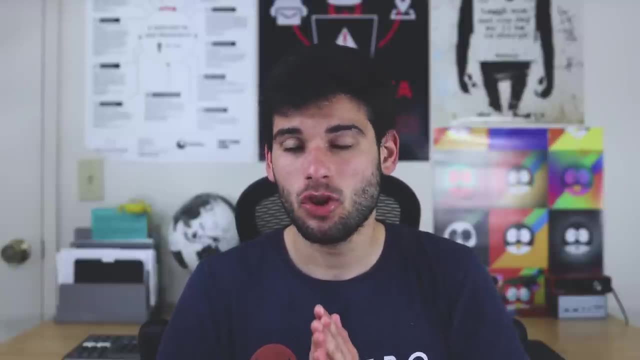 this: your pseudo password is what authorizes elevated privileges, so ensure that is strong as well, assuming it's different from your login password. On a topic of pseudo, you should avoid root login as much as humanly possible and stick to pseudo when you can. As a side note. 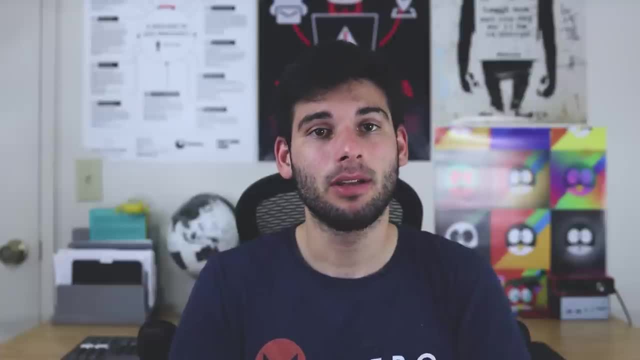 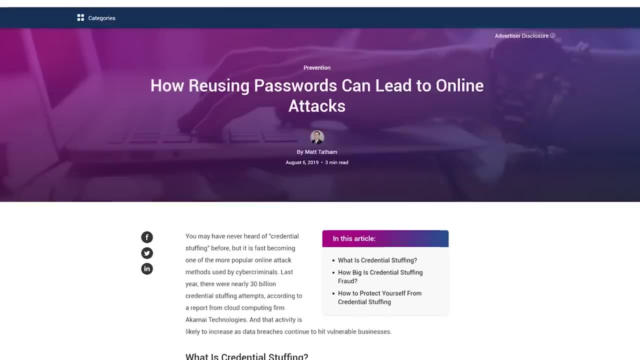 make sure notifications, as well as any widgets and settings toggles, are not publicly accessible on your lock screen. Passwords you use on websites are a commonly left out part of your security. If you use the same or similar password for all your services, one breach can. 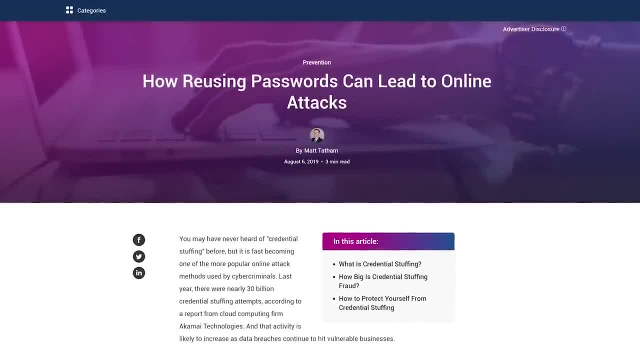 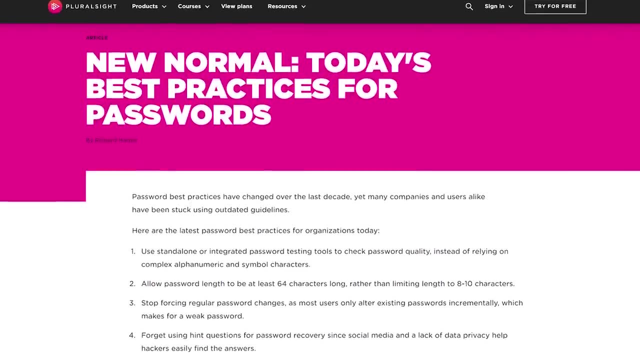 very easily lead to the others being breached since they utilize the same or similar credentials. Make sure- at least in zone 1, that you are using strong and unique passwords. I'll leave a source on what that means and different methods of doing it. Zone 2 will go further into this. 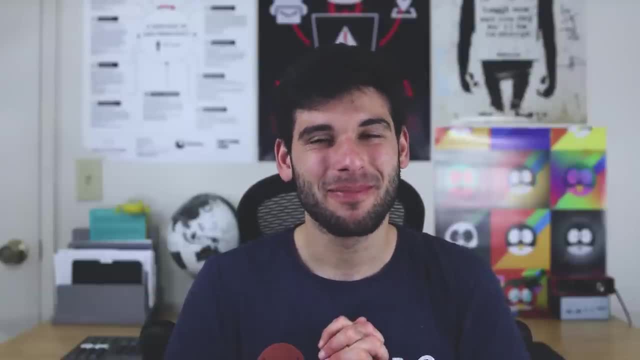 Encryption on Linux is, overall, a pretty happy place to be. Many distros allow you to easily set up locks to encrypt your entire disk, a partition or just your home directory. Ideally, your entire disk is encrypted and if you wanted further file-based encryption. many distros include their own tools to do it, or you can always use something like VeriCrypt. You have a lot of options here at your disposal, making this almost a non-negotiable for your security, to prevent anyone from gaining access to your files by just getting physical access. 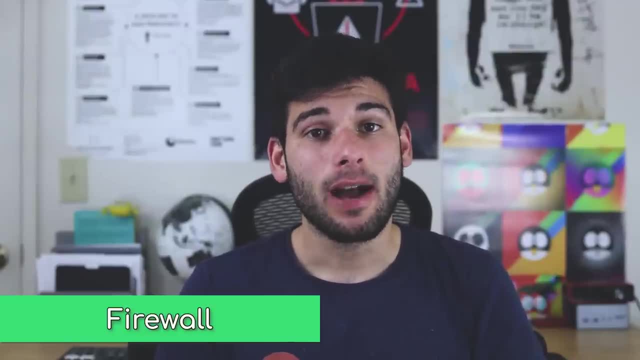 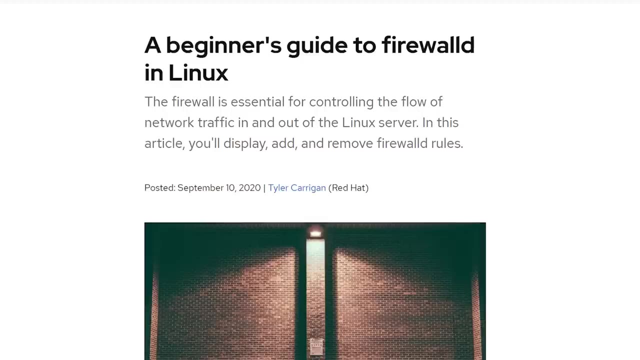 to your machine Up next, you're going to want to make sure you're utilizing a firewall. Linux gives you many options here as well, which can get confusing. but stick with me: IP tables, NF tables and firewalld are firewalls, and they all have different pros and cons. 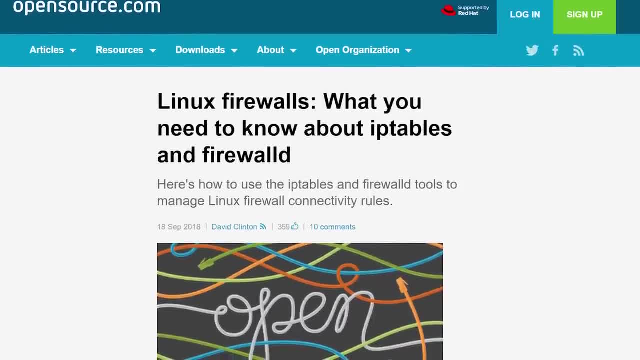 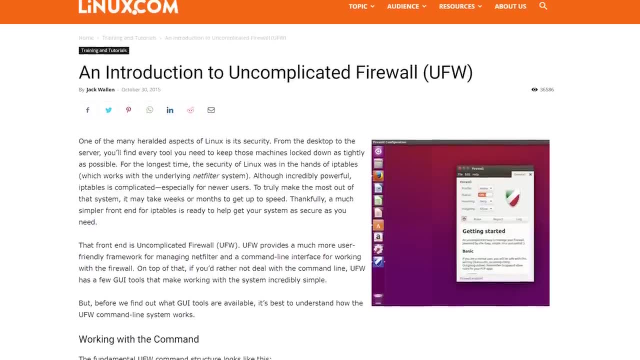 deserving of its own video. We'll include a resource to get you started on that as well. If you're interested in learning more about this, you can click on the link in the description below. However, to keep things simple, we also urge people to check out UFW, or Uncomplicated Firewall, which has an even 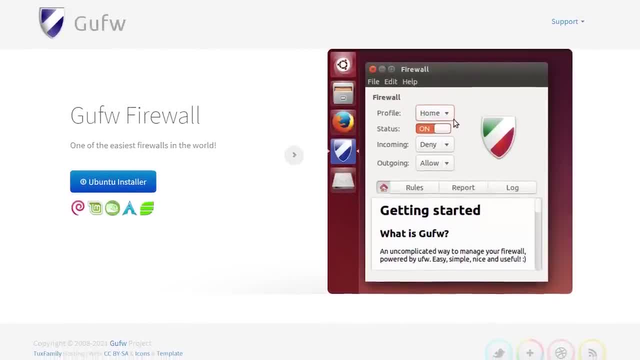 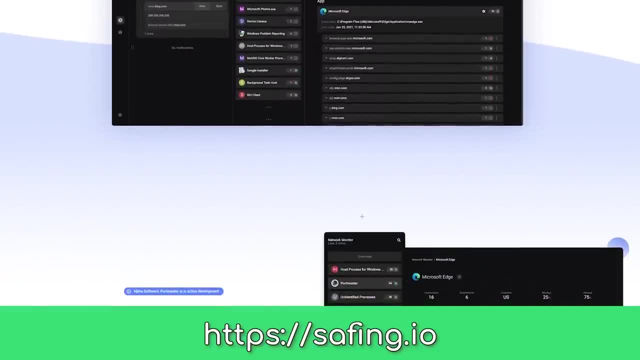 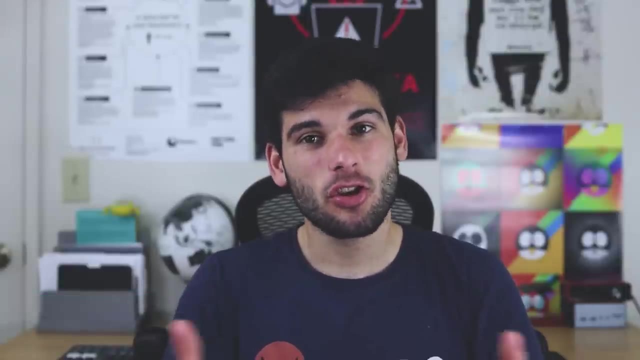 less complicated GUI called GUFW, which is available for most distros. We also recently reviewed Portmaster from Safing that is available on Linux and that may help you in this category as well. Your browser has the ability to track everywhere you go on the internet, Ensuring you. 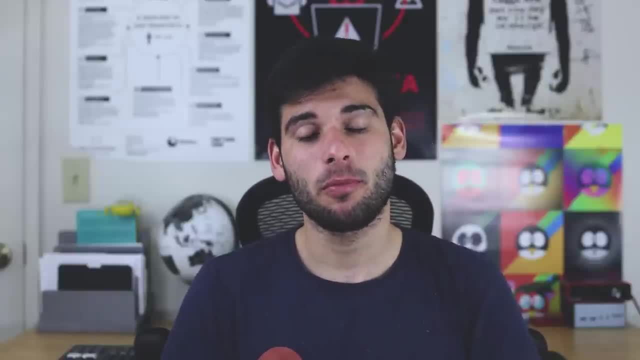 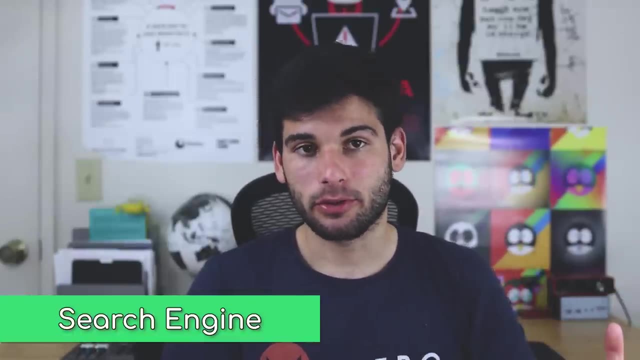 are using something with proven security, and privacy is paramount to protecting your web traffic. For zone 1, we will simply ask you to avoid Chrome. That's it. that's the step. Similar to your browser, your search engine also has the capability of tracking everything you do. 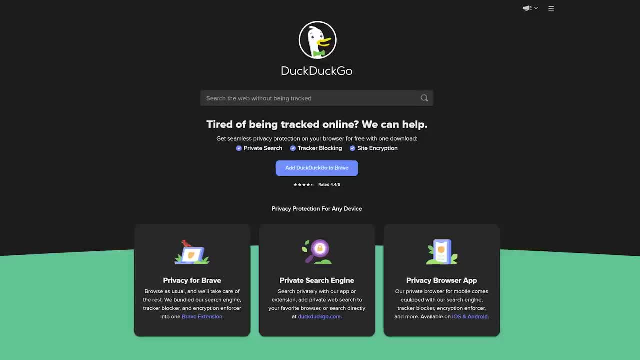 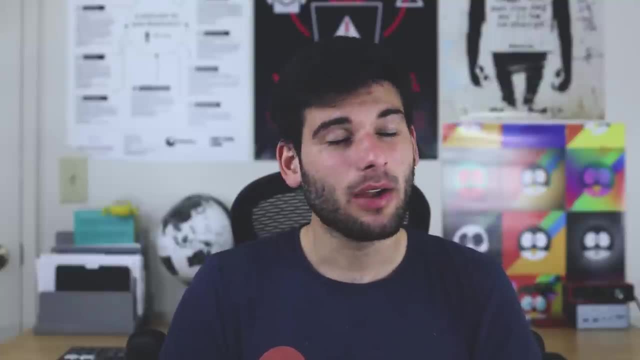 on the internet, which major companies like Google do. The two mainstream recommendations are DuckDuckGo and Startpage, so see if you can implement one of those within your browsers or use something else with privacy and open source in mind, like searchme. Our website's resources page is constantly. 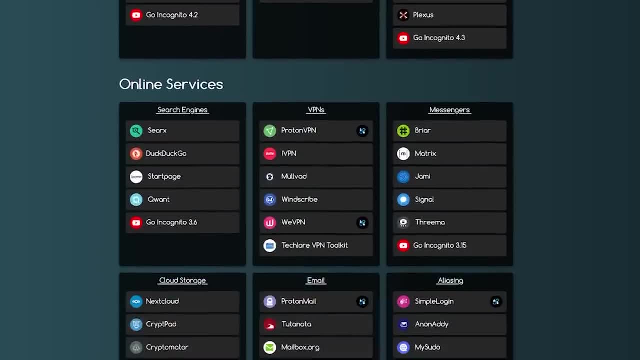 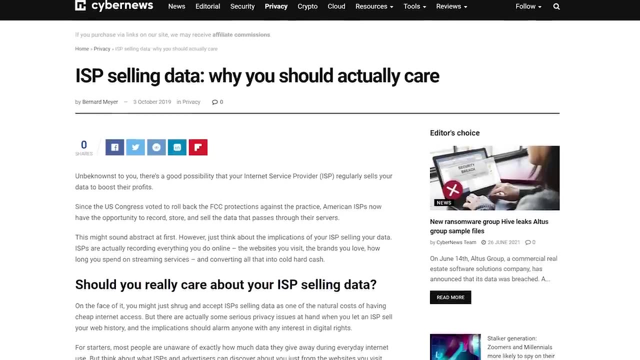 being updated with the newest recommendations, so make sure to keep up to date with that. Your IP is the address uniquely identifies you on the internet, and it's used by websites to track you, not to mention your ISP can harvest all of this data. A simple way to prevent this is by utilizing 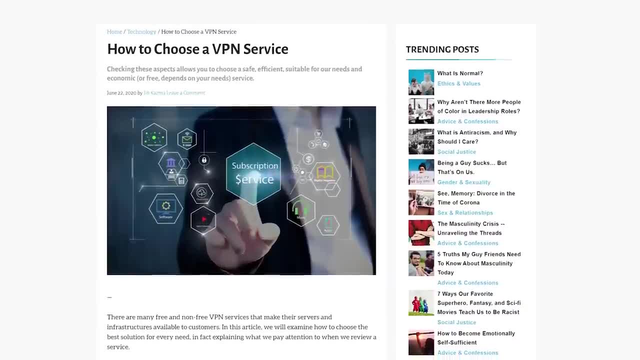 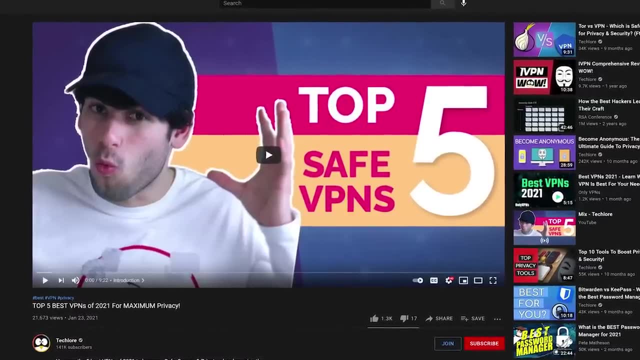 a trusted VPN provider to handle your web traffic. As for which VPN to choose, we do systematic community-driven VPN reviews on our channel. I'll leave our most current top 5 best VPNs video as a card and in the description. We also have all our open source tools on our website, including a chart. 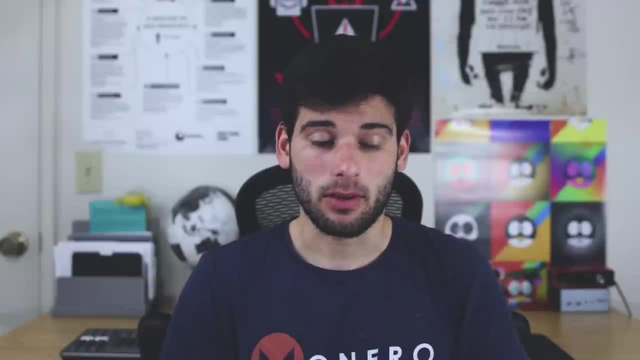 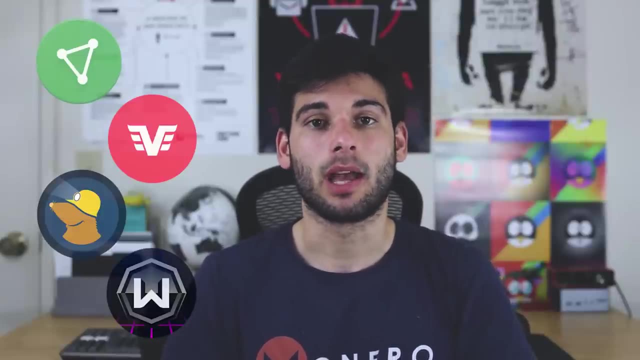 where you can compare different services. At the time of making this video, I recommend ProtonVPN, iVPN and iDubbbz. If you have any questions, feel free to ask them in the comments below. If you want to learn more about these services, you can click on the link in the description to know more. 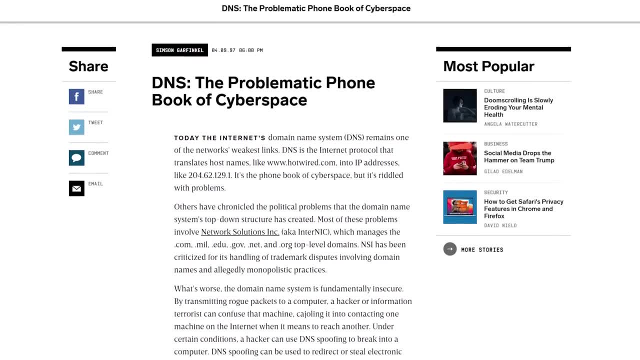 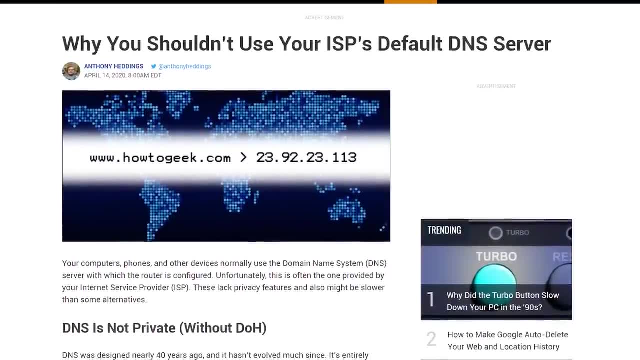 DNS is a domain name service and they're like a phonebook for the internet, directing you to the sites you visit every day. The problem is: most default DNS providers track your browsing, so use a DNS provider with privacy in mind If you're using a VPN service. 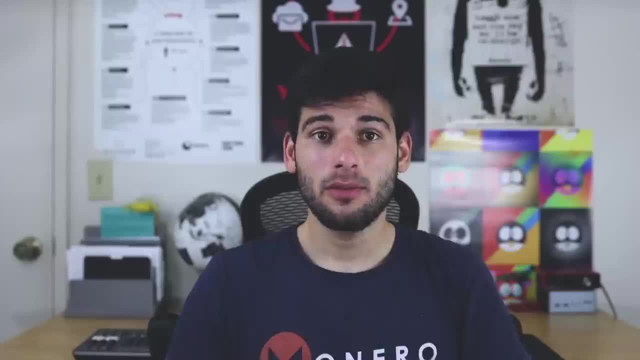 it likely uses its own DNS, meaning you don't have to worry about this. If you aren't using a VPN, check out the DNS options on Privacy Tools IO and manually set them on your computer. Instructions on how to do that are in the video description below, If you haven't already done so. 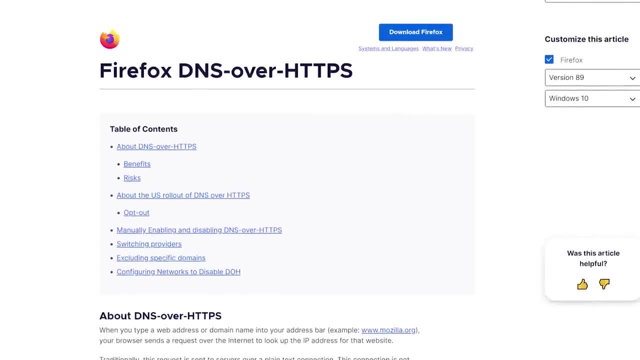 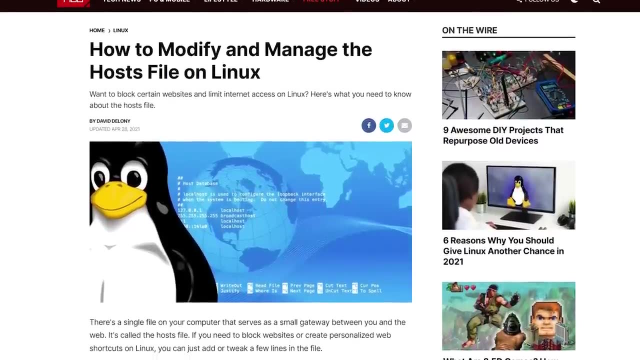 how to do that are below. You can also use some browsers that utilize other DNS improvements if you choose to. Lastly, you can use a host file to prevent certain naughty domains from being accessed altogether. This is broad, but less is almost always more when it comes to security and 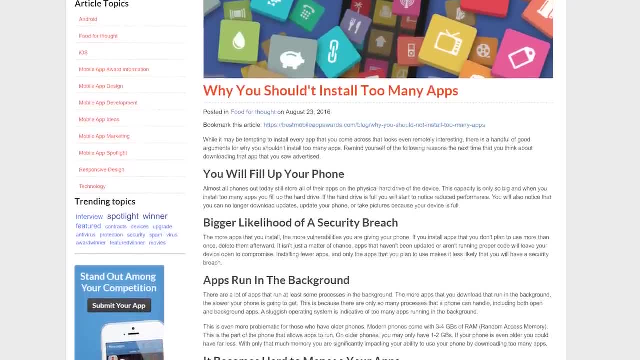 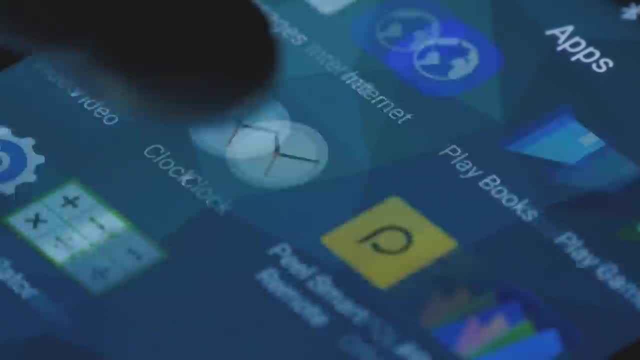 privacy. Each additional program and setting you utilize increases attack surface and the possibility of abuse with your personal information. If you're a person with a never-ending list of programs that you mostly never use, they're likely not just doing harm in the background with your data, but also negatively impacting things like storage space. 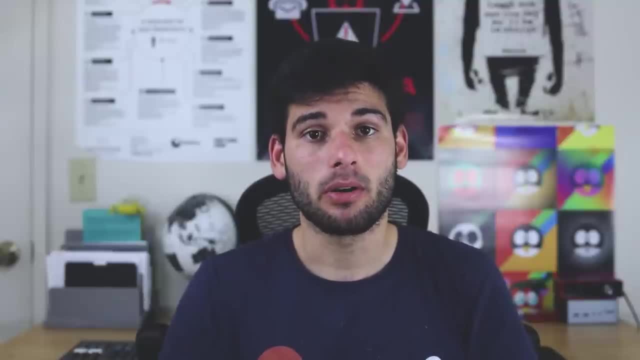 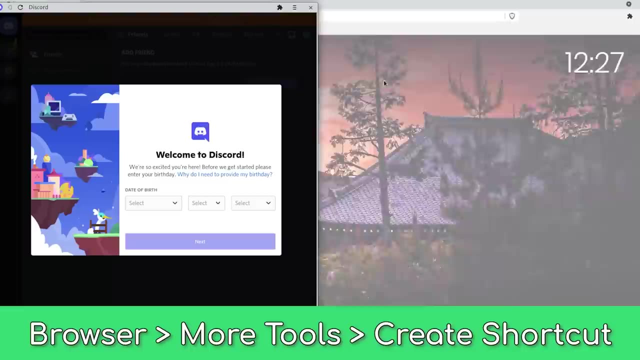 and power consumption, so just delete them. Or, for the bloatware, uninstall as much as you can. Some programs, like Discord maybe, have progressive web apps, so if you can utilize the web application within your browser to function like the program, it's a great way to separate the. 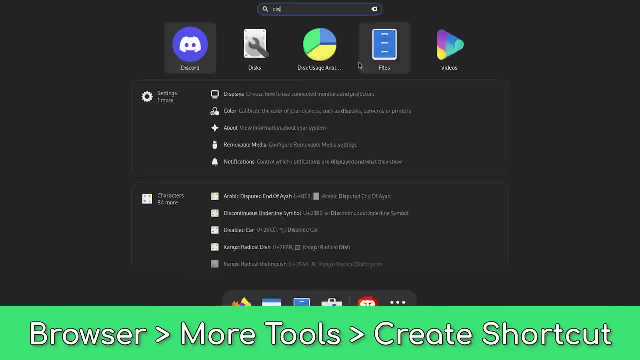 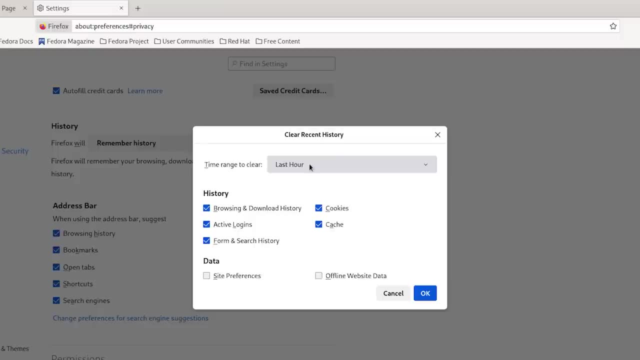 program and keep it within your browser, which is typically safer and gives you a bit more control Outside of programs and settings. try to frequently clear data you don't need, like old system logs, temporary data and other data that you don't need. If you have a lot of data that you don't need, 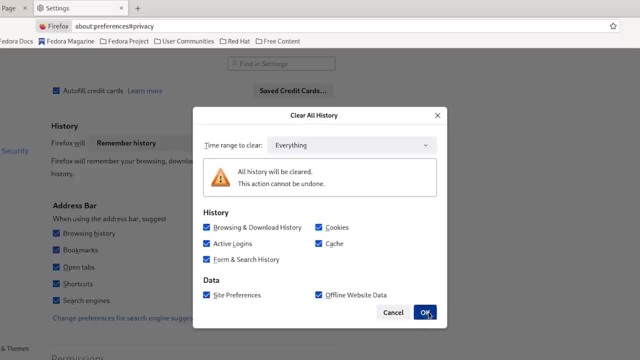 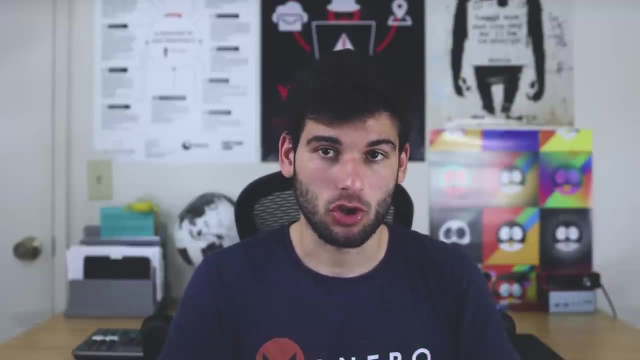 like browser cache, history, cookies and any sensitive data that doesn't need to be on your computer 24-7.. Free and open source, or FOSS, is another important aspect of this, and we'll talk about that more in section 2.. Bleachbit is a wonderful tool you can use to help in this. 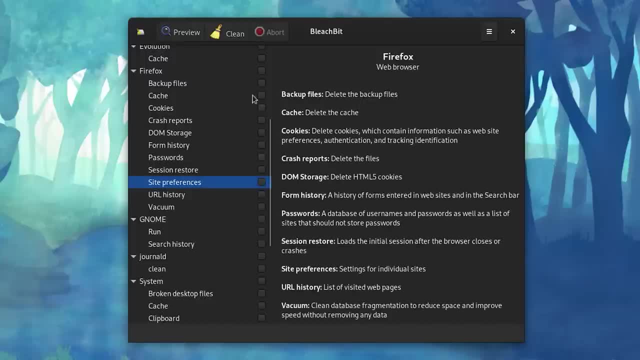 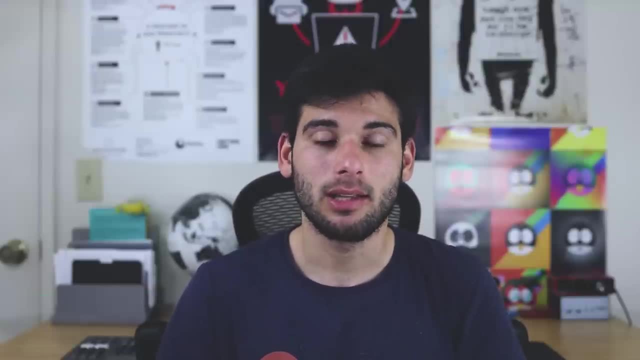 category, though, proceed with caution, as it can cause damage if you're not careful. Tying into minimalism, there are lots of settings on Linux and its programs you may never use that are pointlessly collecting data about you. The general rule of thumb is: if you're not using it. 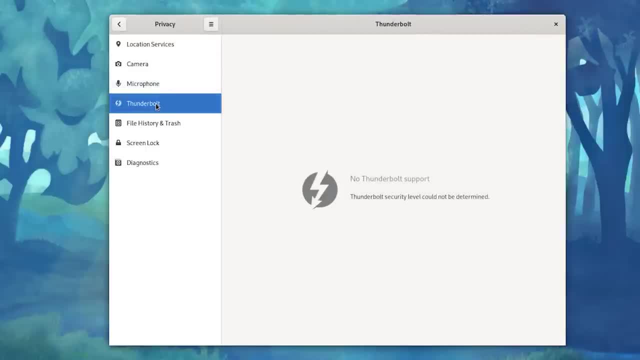 turn it off. Make sure to be thorough and if you're not using it, turn it off. Make sure to be thorough and double check every setting inside your operating system and don't forget to go through each individual program's settings to ensure nothing is. 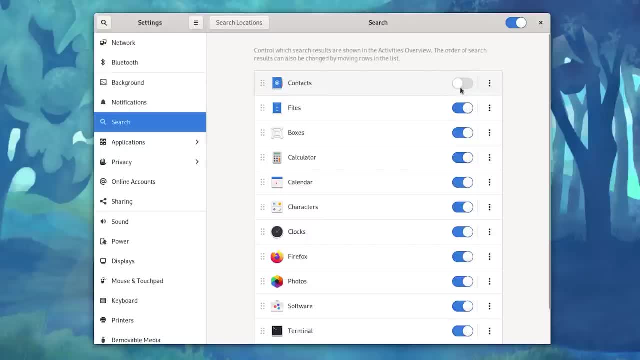 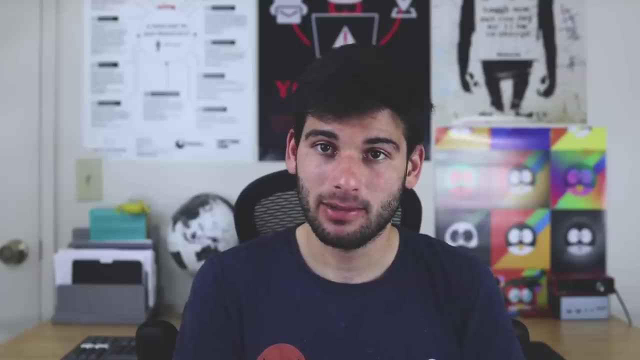 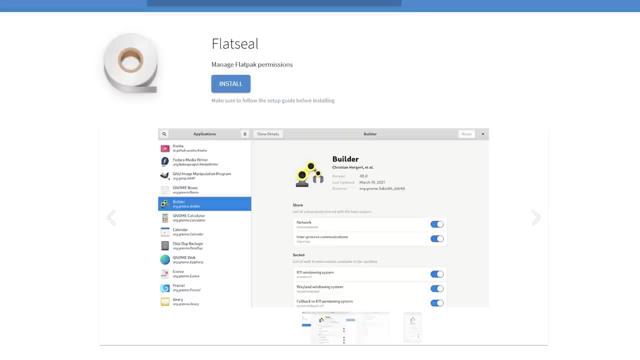 needlessly tracking you within the program. On a similar note, program and OS permissions shouldn't be taken lightly either. Think twice before giving a program elevated permissions on your operating system and consider using something like FlatSeal with your FlatPaks to fine-tune permissions on a program basis. We'll talk more about this in Zone 3.. 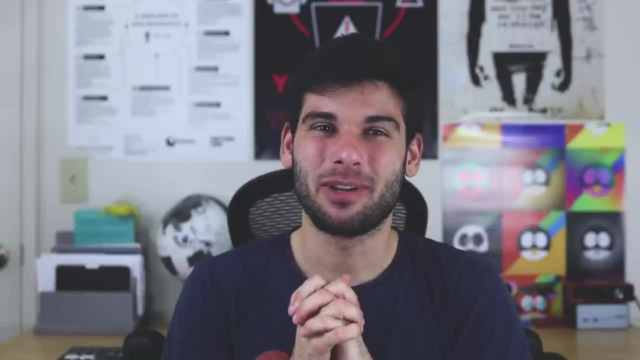 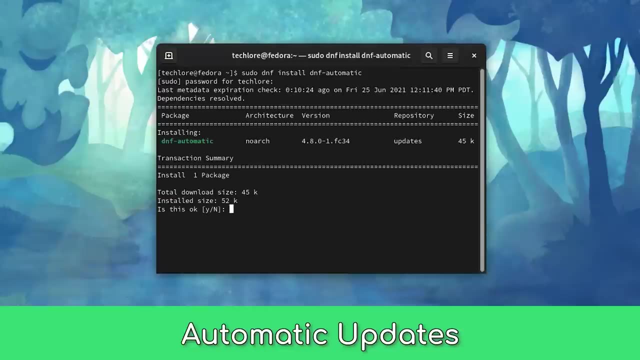 I don't know why the Linux community doesn't use FlatSeal. I don't know why the Linux community is one of the most stubborn communities regarding updates. Well, I kinda do, But in 99% of situations, automatic software updates are good and beneficial and patch urgent exploits For most people. 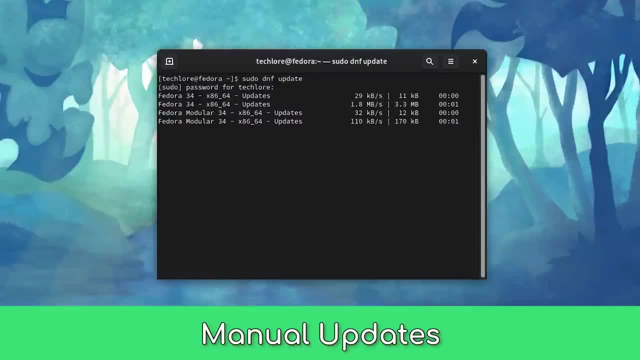 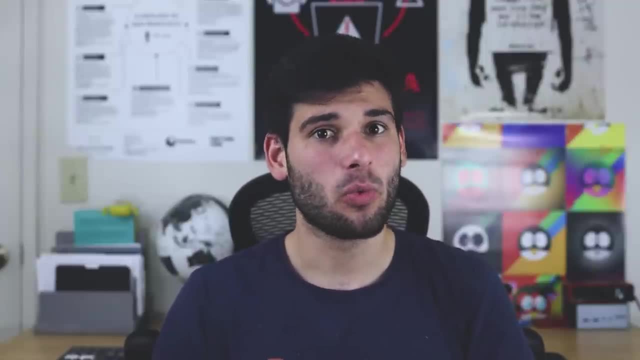 we recommend utilizing automatic updates or doing it yourself frequently, no less than once a week. Yeah, that's it for Zone 1.. Everything here we recommend the entire world implements as it doesn't really impact convenience and is almost universally better for your privacy and. 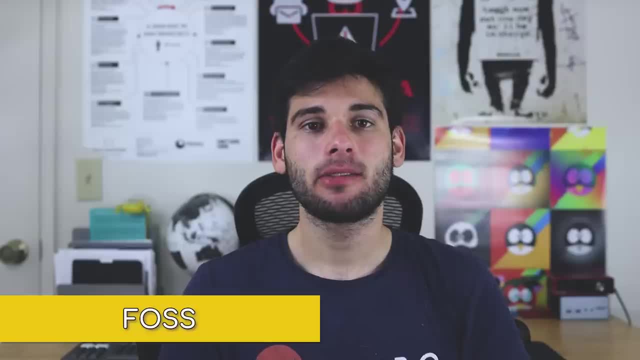 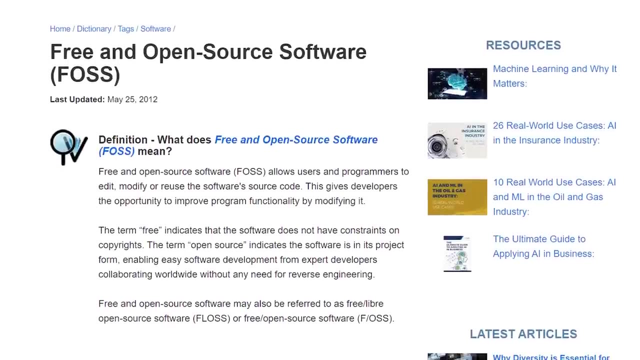 security. FOSS stands for Free and Open Source. This means the software's code is publicly accessible to the community. This ensures you can verify the security and privacy behind the software. We have a video covering this a bit more thoroughly. In general, I'd advise moving. 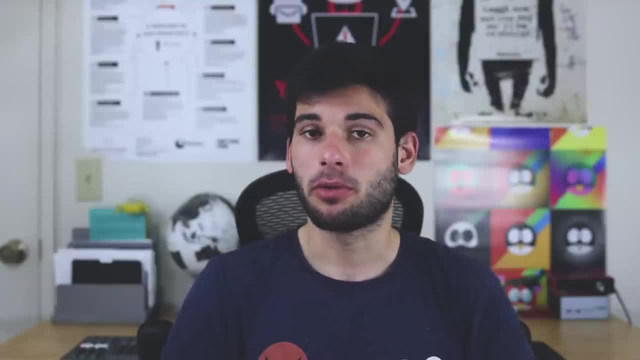 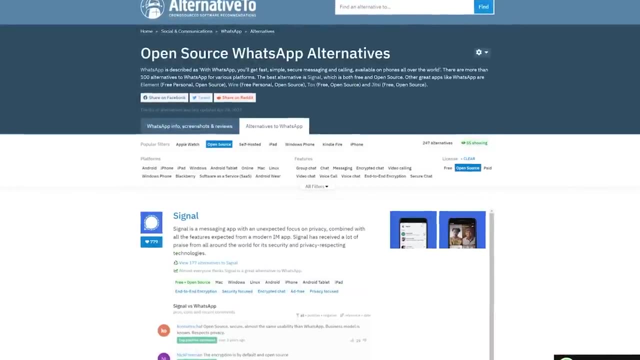 from proprietary to FOSS programs as much as possible. Just go through your list of programs and type each of them into Alternative2.net with the open source filter and see if there's something you can reasonably switch to. FOSS will typically honor you and your data better than 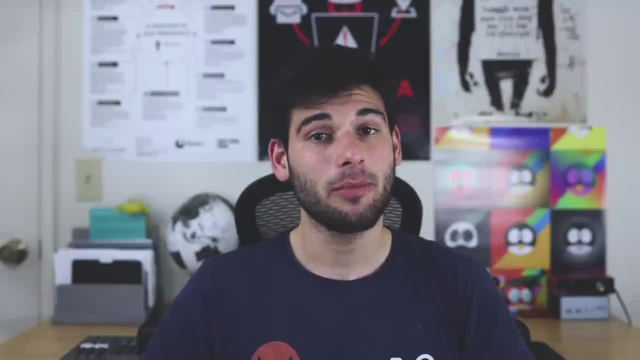 proprietary software. FOSS will typically honor you and your data better than proprietary software. FOSS will typically honor you and your data better than proprietary software, And you are on Linux, where the FOSS community is the strongest, so make sure to take advantage of that. 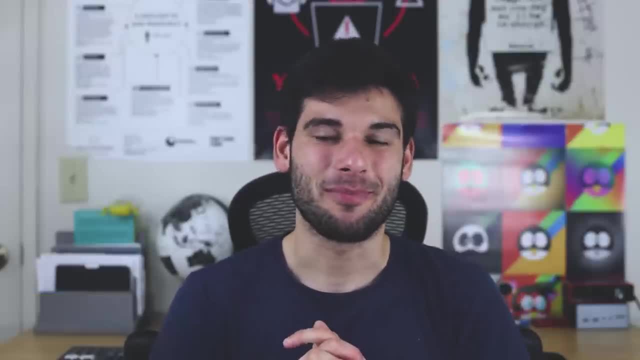 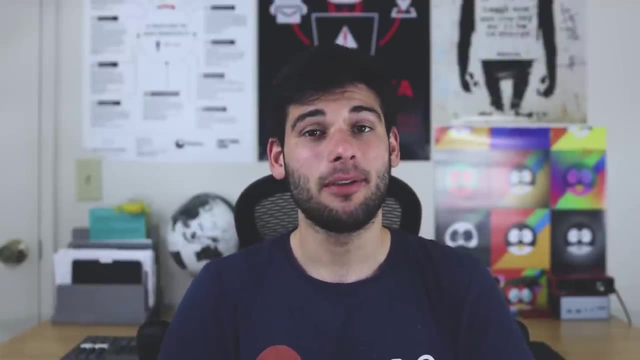 Your computer is, ironically, used less for communication than you might think, at least in the context of direct contact with another individual or individuals With email. it's recommended to keep email in your browser to add an additional safety layer between an email and your operating system In regards to what email provider to use. 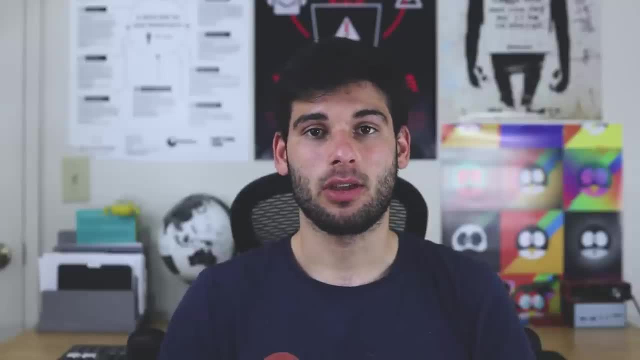 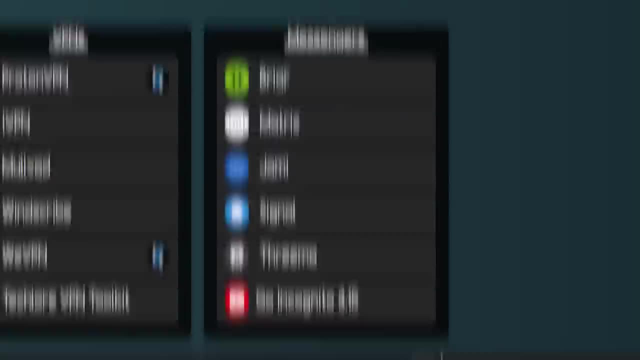 we have a nice video on that you should go watch. With direct messaging first, I recommend switching to something built from the ground up to protect you, like Signal or another Messenger listed on our site's resources page. Or we recently just put out a Top 5 Messengers video as well. you should go watch If you're stuck using something like. 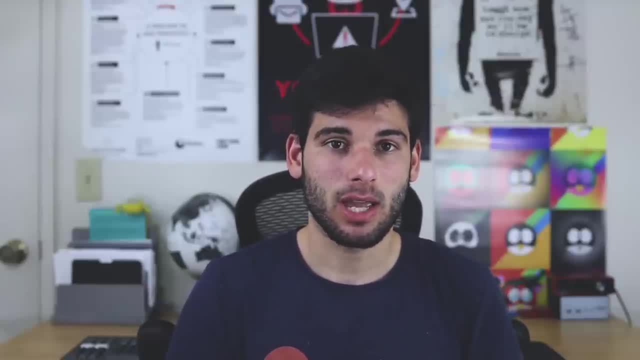 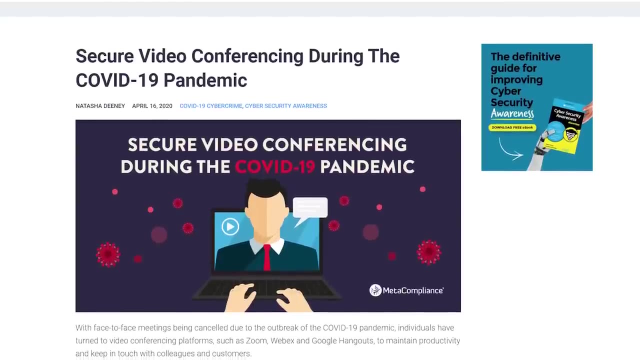 Facebook Messenger or WhatsApp. enable end-to-end encryption where you can, and try to keep the program off of your computer as well, keeping them inside your browser instead. Thanks to the pandemic, video conferencing is the next big thing, and like direct messaging. 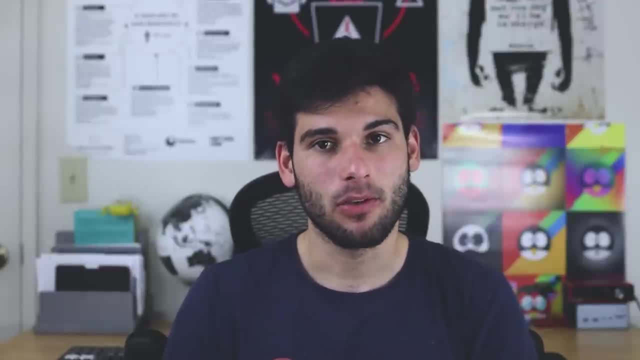 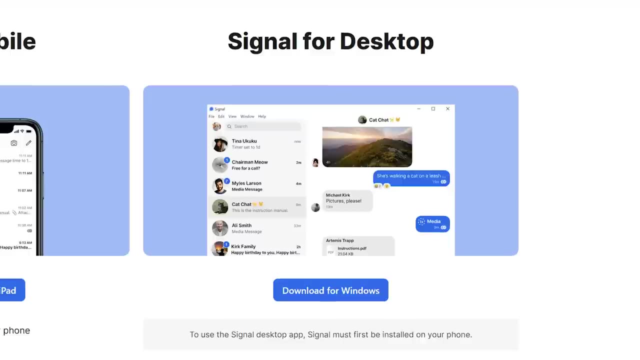 the first goal is to move to things that naturally respect you. Jitsi, Kallax Meet, which is an instance of Jitsi, and BigBlueButton are all good alternatives to Zoom, Skype and others. Oh, and Signal finally got desktop video support, so that is also a good option. 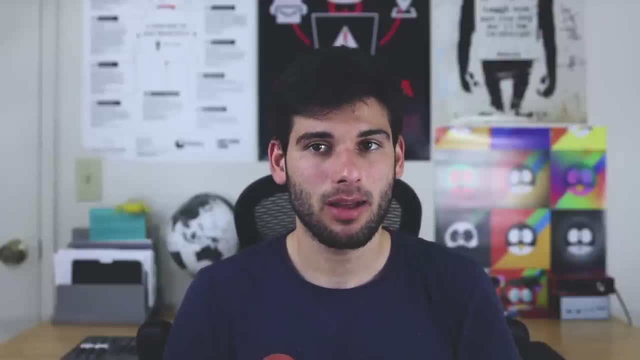 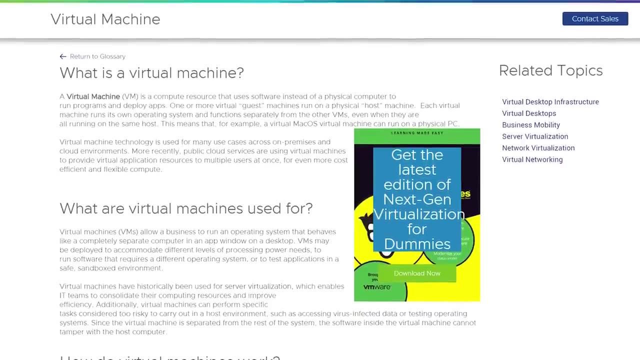 Finally, like direct messaging, if you're stuck on a not-so-great platform, the goal is to keep it inside your browser when possible and avoid using the program. We'll talk about virtual machines later in this video, which are also good tools for invasive programs when you need them. 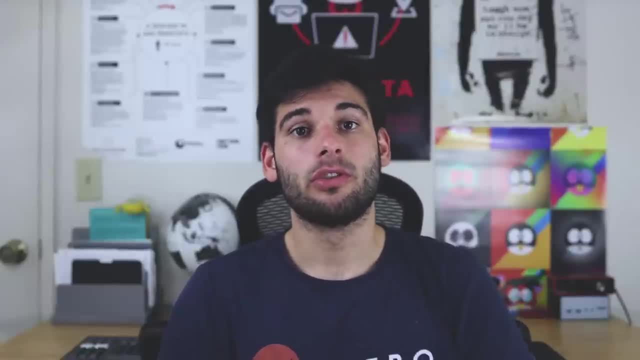 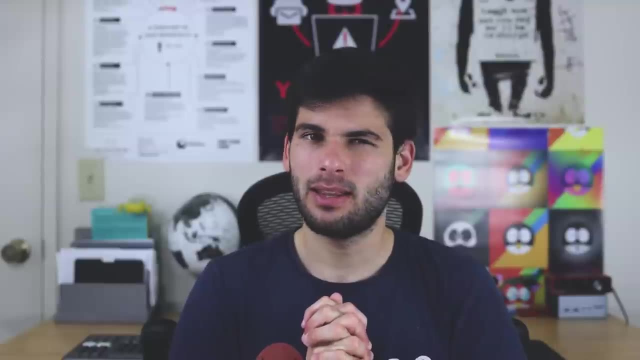 Avoiding Google is a great step for controlling your data, as Google is not a privacy-friendly company whatsoever. Use Flash For Zone 2,. we normally encourage the avoidance of Google, but in this Linux guide we assume you're a bit more advanced, so we're actually going to recommend the full deletion of. 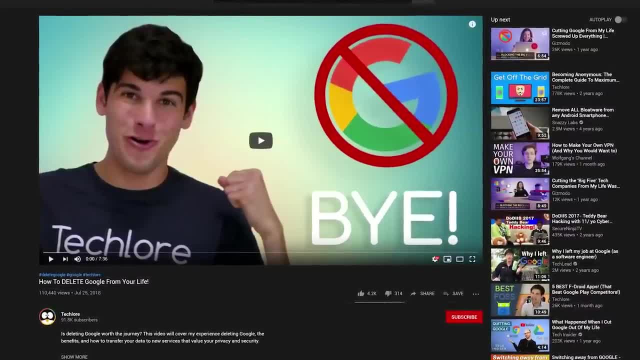 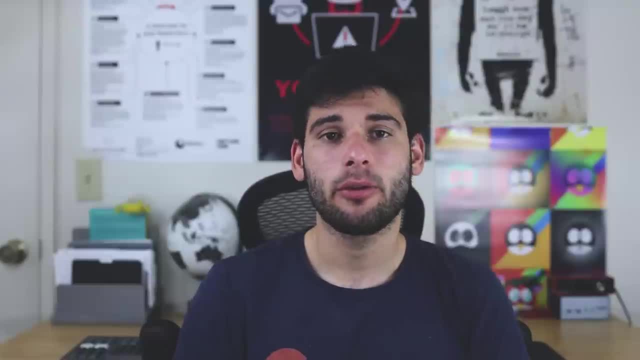 Google. We have a video that breaks down this journey more thoroughly. we recommend you check out Outside using strong and unique passwords, which we covered in Zone 1, where and how they're stored can be incredibly important as well. Password managers are a commonly recommended way to go. We've covered which ones to use in. 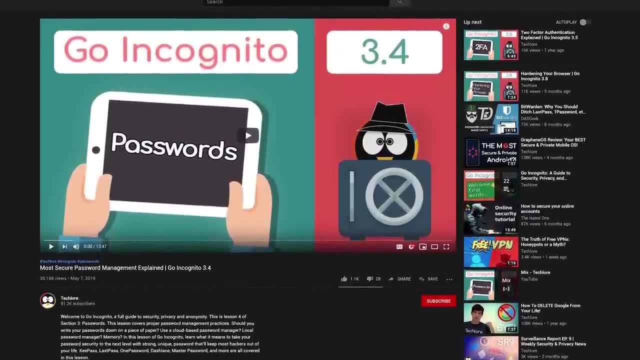 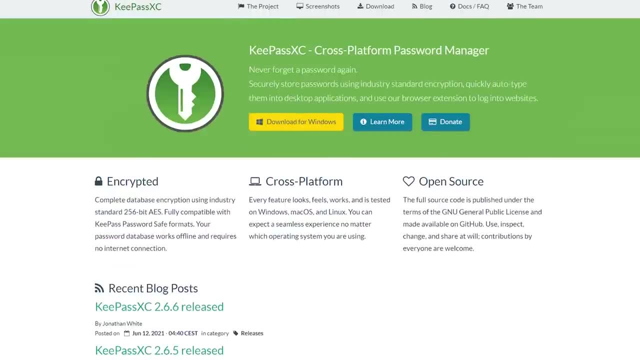 the lesson of Gointotteneo, so check that out for a long answer. In short, avoid storing your passwords within your browser. If you want simple cloud-syncing between your devices, check out Bitwarden If you want a more DIY password manager. 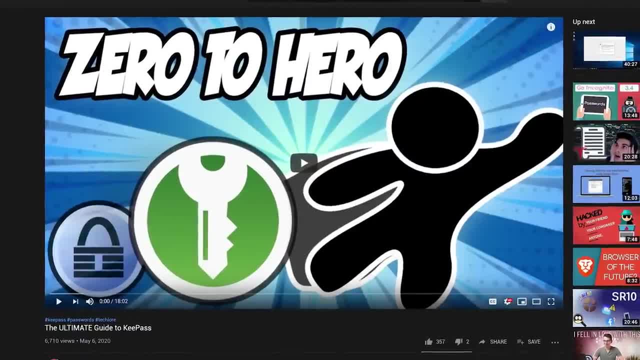 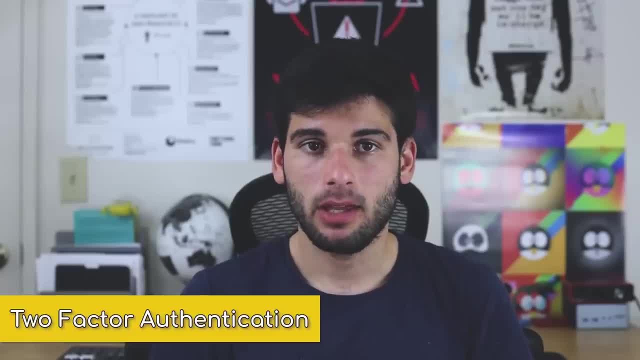 there's KeePass. We have a whole guide to KeePass on our channel for those who want to learn how it works, as well as a comparison video between these two fantastic open-source password managers. Beyond having a strong password, implementing two-factor authentication is arguably just as important. 2FA combines 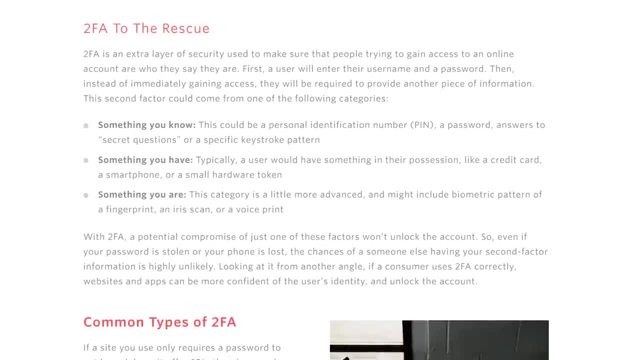 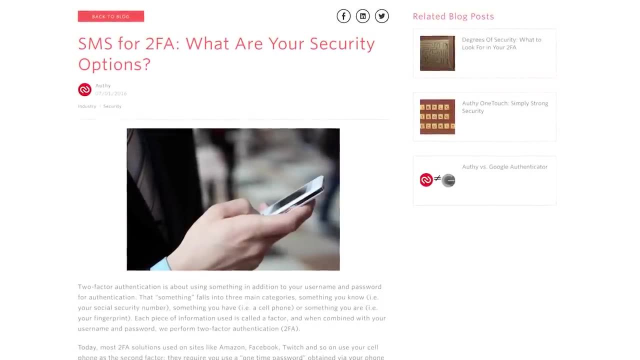 something you know, a password with something you have, like a code generated locally on a separate device. At the very least, SMS-to-FA, which are those texts you receive with a code, are better than nothing. but there are a couple issues with SMS-to-FA, like the risk of SIM. 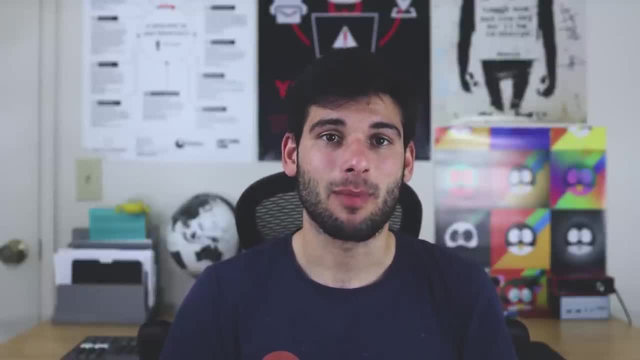 swapping. The better and more recommended option is a local authenticator app on your phone that uses a QR code. Not every site supports this, but many do, so look for it and use it instead of SMS when you can. If you want FOSS recommendations, Android has Aegis. 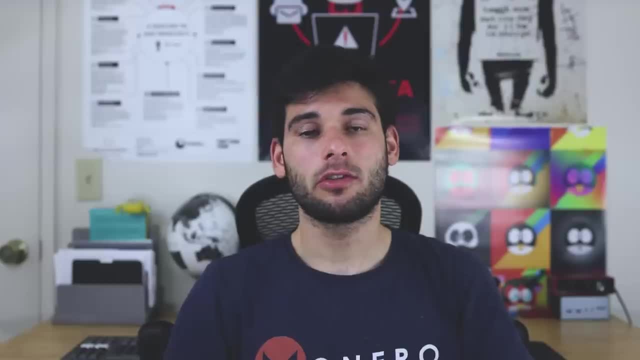 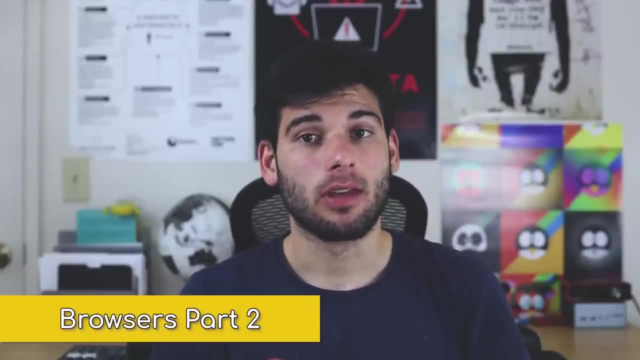 and for iOS there's Raivo Authenticator and Tofu. It's also worth mentioning there are hardware as well which can be used for sudo with a bit of work. Part 2 of browsers is to take things to the next level. I'd recommend sticking to strictly. 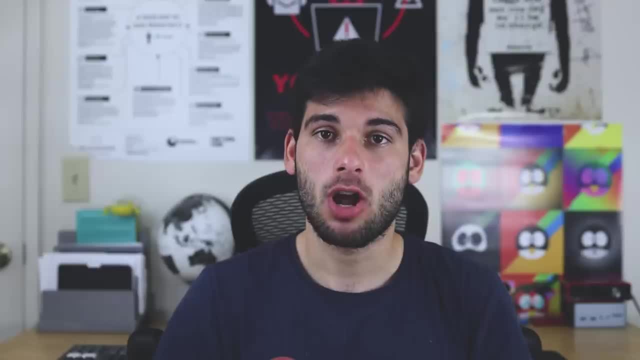 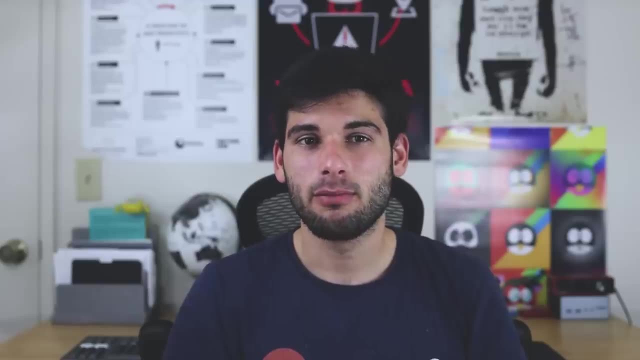 open-source browsers like Tor, Firefox, Brave and Chromium, and properly hardening and configuring each browser for the absolute best safety. We cover Firefox. hardening in Go, Incognito and Brave mostly requires just basic settings, toggles, as it does much of the work for you. 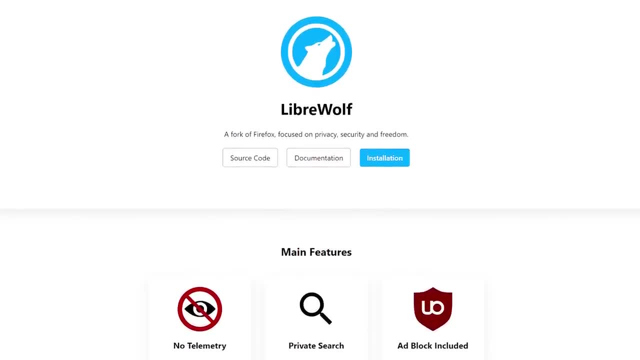 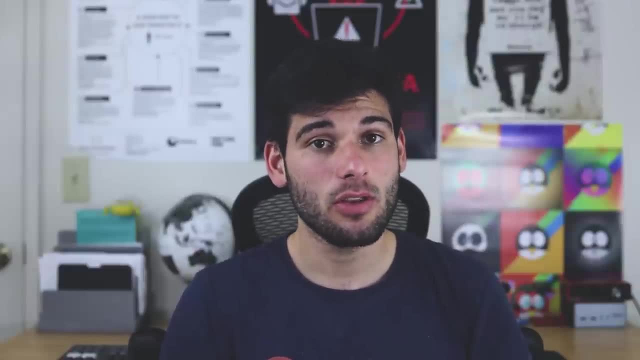 out of the box. LibreWolf is something you can check out. to simplify, Firefox and Tor should not be messed with outside the basic safety sliders. No matter which browser you choose, you should avoid installing extensions you don't need, as these can be some of the most problematic areas when it comes to your browser. 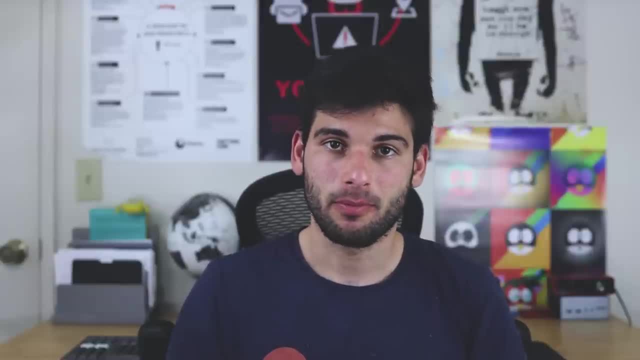 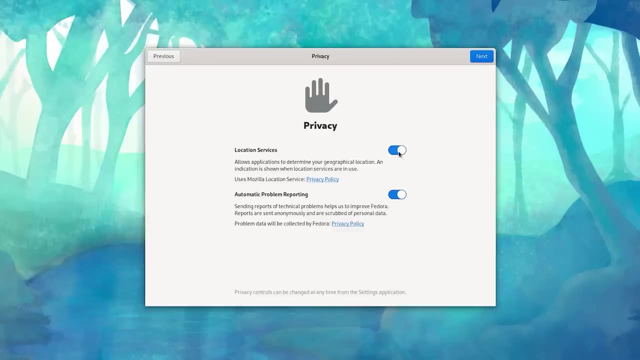 Radios apply to anything that gives off a signal on your computer. This means predominantly WiFi, Bluetooth and GPS. We'll cover the more extreme solutions in Zone 3, but for Zone 2, try disabling Bluetooth and location services when they're not being used. 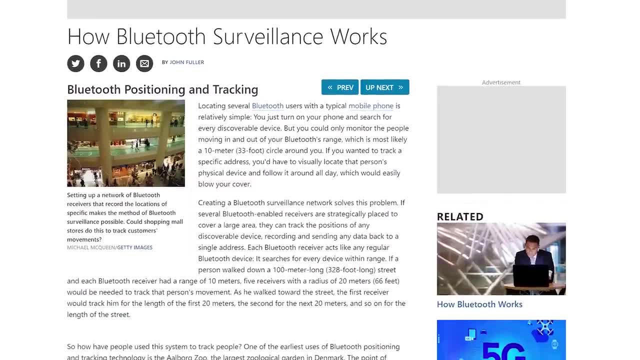 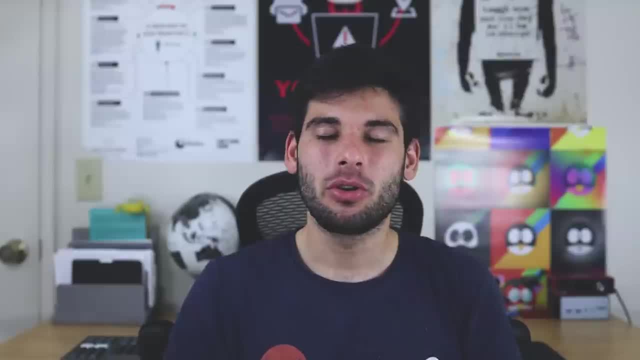 Bluetooth for one can be an insecure protocol, not to mention it's an instrumental tool used to track your movements. This is a smaller concern on a computer, as it's likely not traveling around town alone, but it's still good practice. The last radio you should be aware of is WiFi. 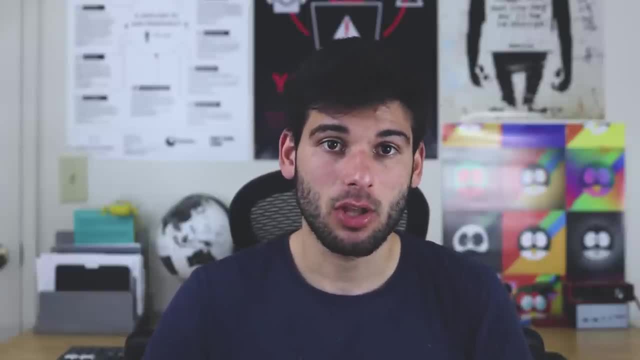 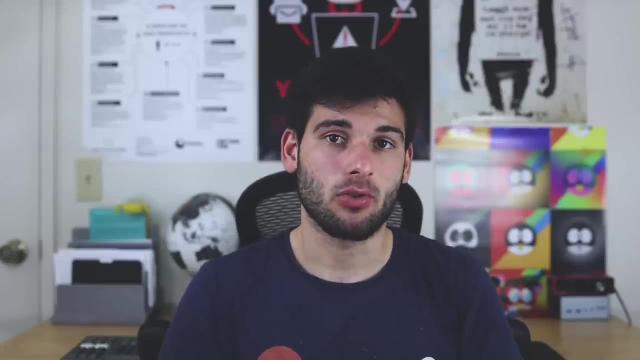 Your device broadcasts a unique ID called a MAC address, which can be used to track you. We covered how that's done and how elaborate it can be in Go Incognito. In short, consider randomizing your MAC address. MAC Changer is an easy and convenient tool that does this for you automatically. 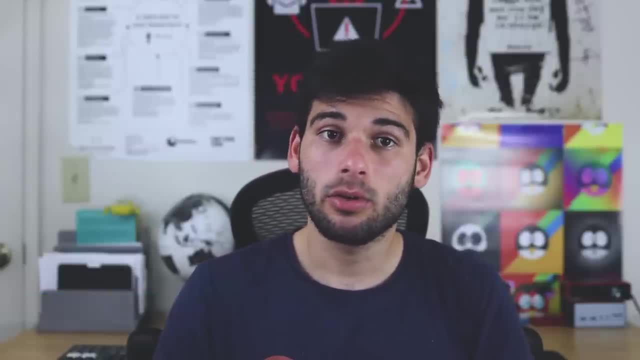 You can create several user accounts and use these to compartmentalize or separate different aspects of your life. Maybe you have a business account, a school account, a dating account and then your personal account. The options are limitless. The goal here is to separate. 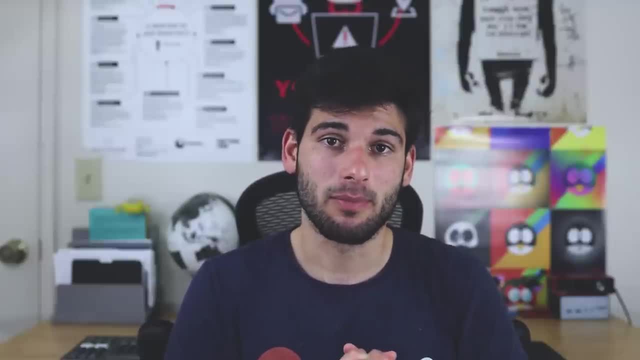 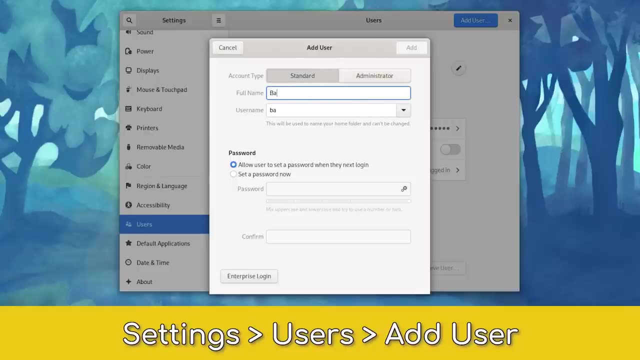 aspects of your life that don't need to be intermixed, for both privacy and security benefits. Additionally, for those who want to go above and beyond, you can have an admin account and then a standard user account and stick to only using the standard user account for your. 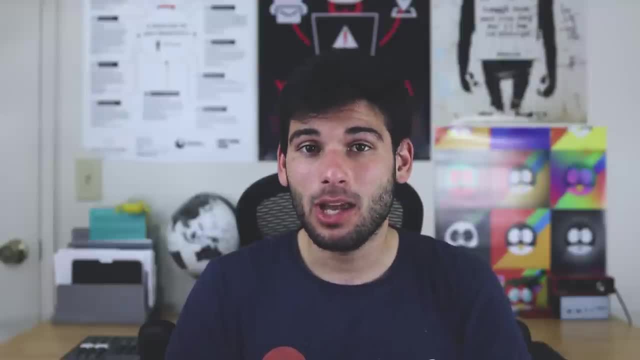 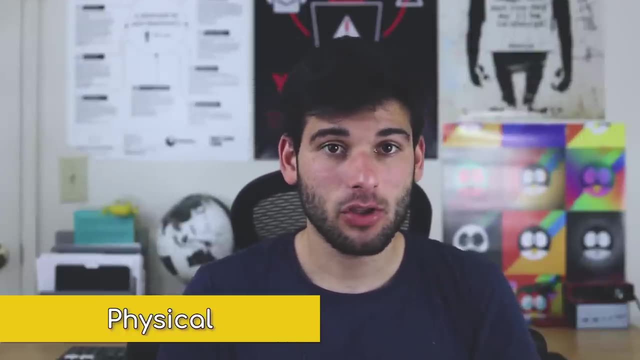 daily usage. as a security perk, This prevents any rogue applications, malware or anything else from utilizing that administrative access to damage your system. Some extra tips in regards to physical protection of your computer. First, lock down your BIOS through its basic settings and maybe consider swapping it with something like Coreboot. 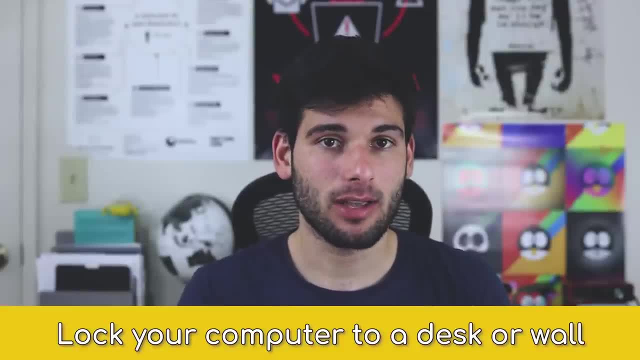 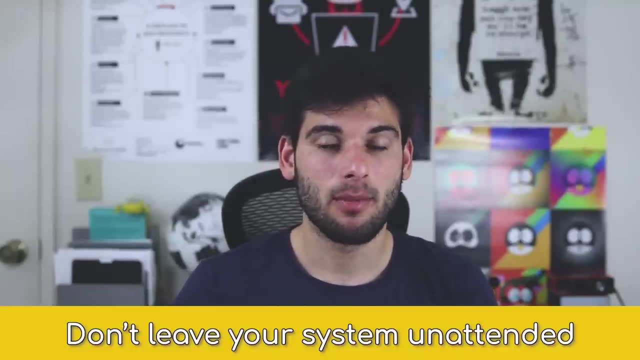 if you're able to Consider locking your desktop or laptop to a desk or wall, if this is an option. I'll leave some products below. Also, don't leave your system unattended, especially in public. Make sure it's always with you. and if you're forced to leave your system unattended, 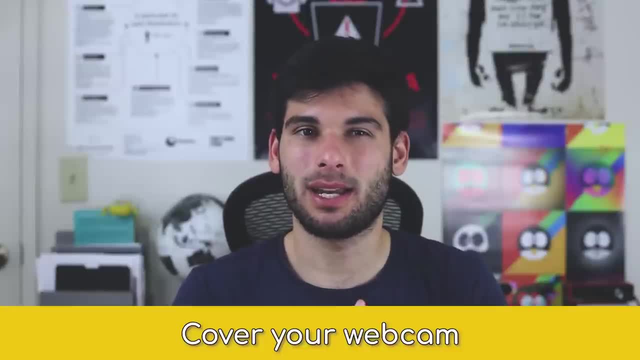 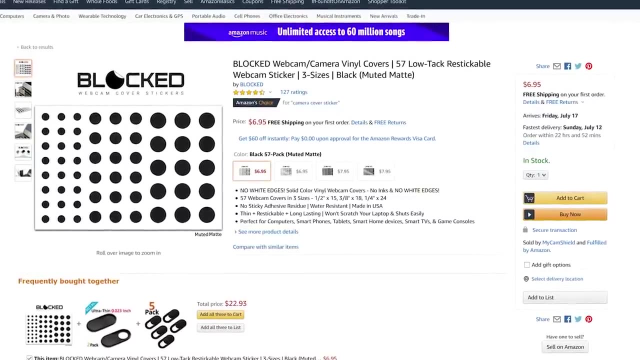 make sure you're logging out. Next, most people are aware of this one, but covering your cameras can prevent that camera hack where someone spies on you through your camera. If you never use your cameras and don't want to just use tape, A nice. 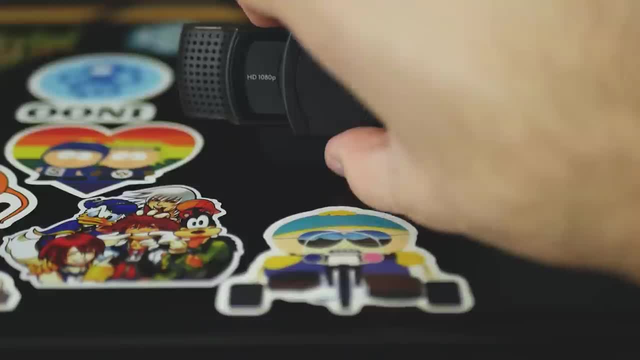 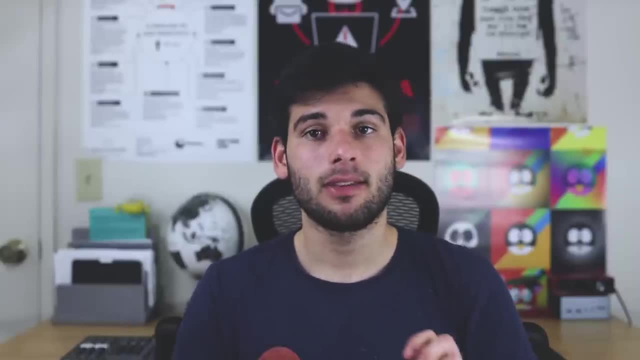 thing with desktops, though, is they normally don't even have a webcam, like laptops do, so you can instead rely on an external webcam with a great amount of peace of mind once it's completely unplugged from the system. The last step for Zone 2 is utilizing a privacy. 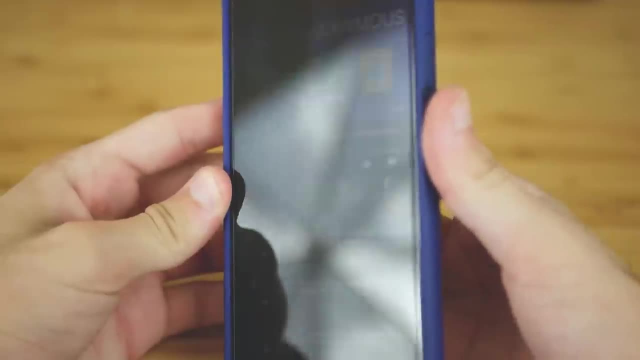 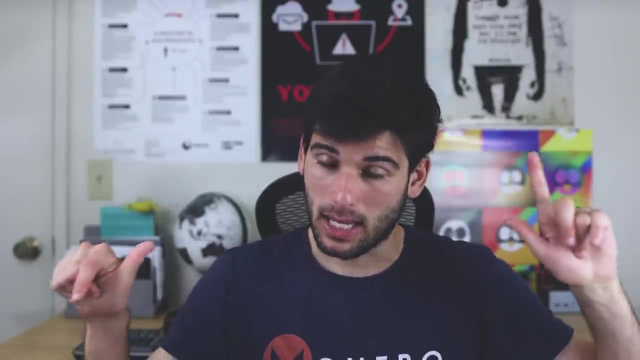 screen protector. These make it so it's very difficult to view your device's screen from side angles, protecting your personal information from snoops and shoulder attacks. I'll leave a link in the description of some privacy screen protectors. I cannot recommend them more. 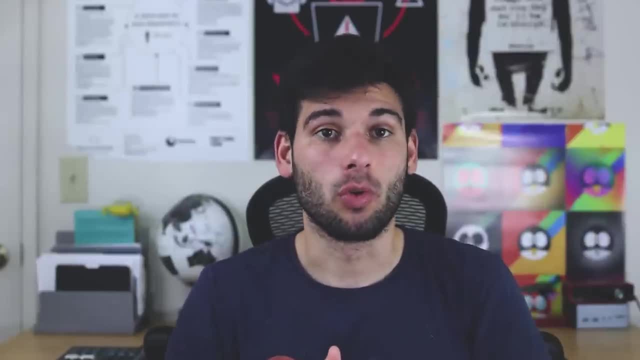 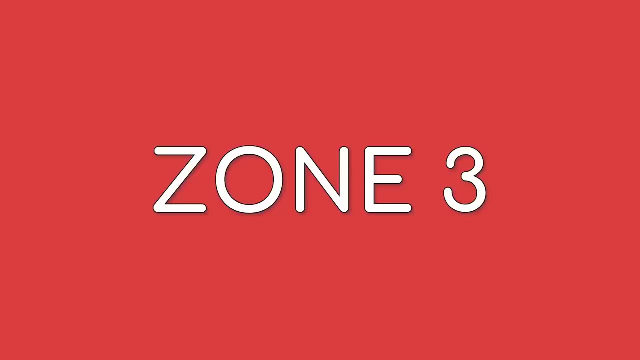 and the peace of mind they give me in public. And that's gonna wrap up Zone 2, where we've accomplished a hell of a lot, but there's still more things to do in Zone 3, so get ready, We're gonna kick off Zone 3 by talking about sandboxing, which, as the name implies, 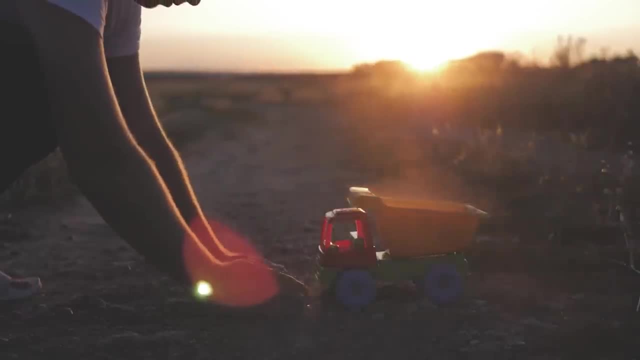 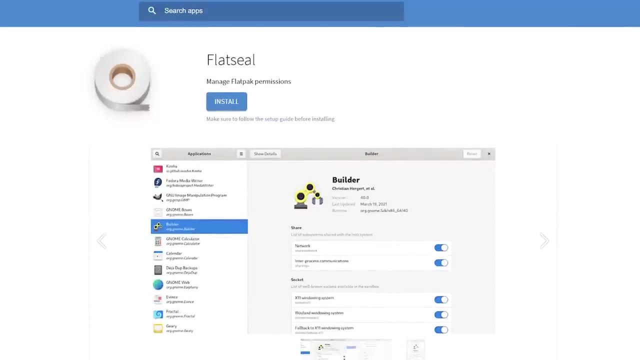 is a little play zone to add an additional layer of security away from your main system. If you want to keep things simple, flat packs are very convenient ways of installing programs and you can use flat seal to handle permission management, in addition to some of the sandboxing. 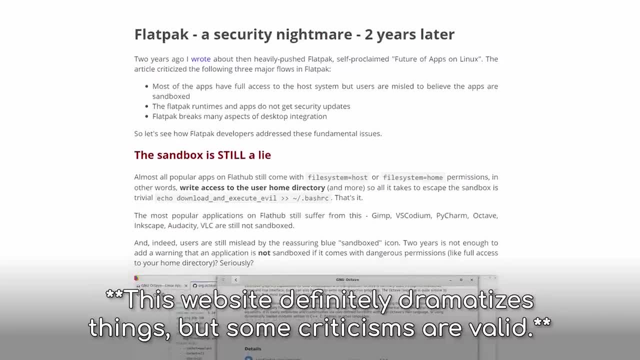 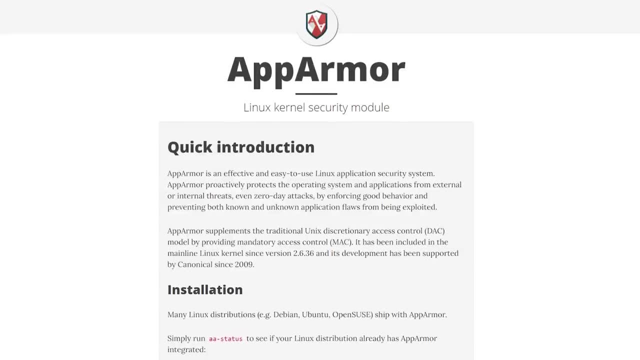 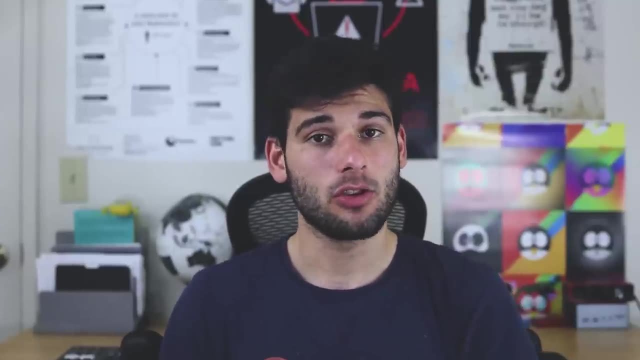 benefits of flat packs. You should be aware there are some criticisms of this approach, but it's still, overall, a solid option. From there, you should consider taking a look at App Armor and FireJail, two other solutions at your disposal to sandbox different aspects of your configuration. FireJail Isolation provides. 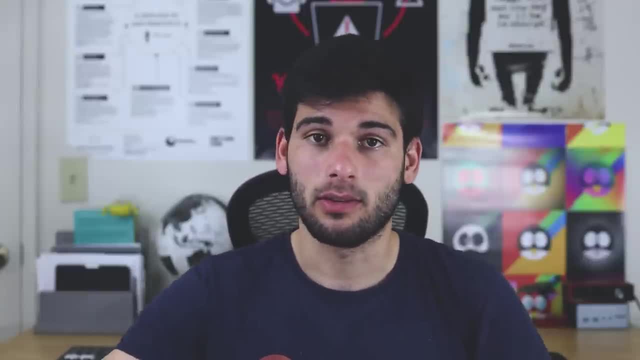 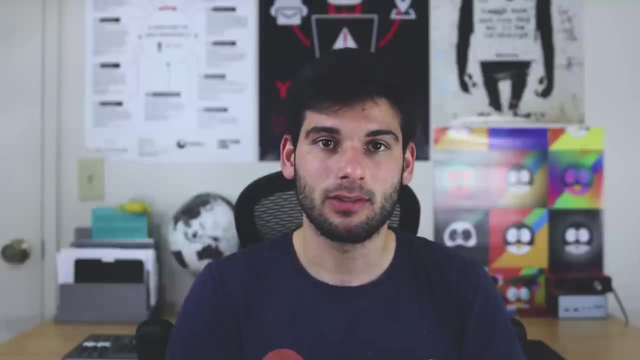 an application, a sandbox, to do whatever it wants while protecting the rest of the system. App Armor technically doesn't provide any sandboxing, but it's still a valuable tool in limiting what parts of the system an application can access. If these two options are too complicated for you, flat packs take you pretty far, So if you're looking to get a, 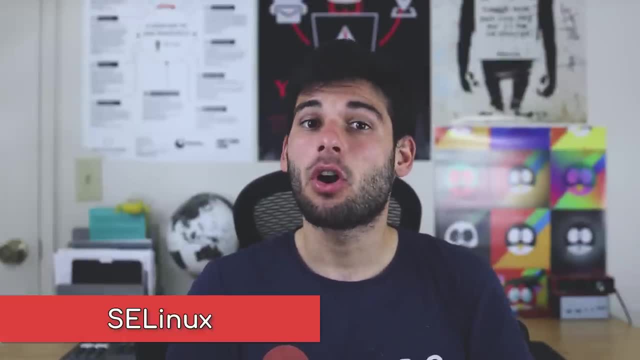 new system. you should consider taking a look at App Armor and FireJail From there. you should consider taking a look at App Armor and FireJail. Before we get into hardening Linux, it's important we talk about SELinux. SELinux stands for Security Enhanced Linux and, as the name 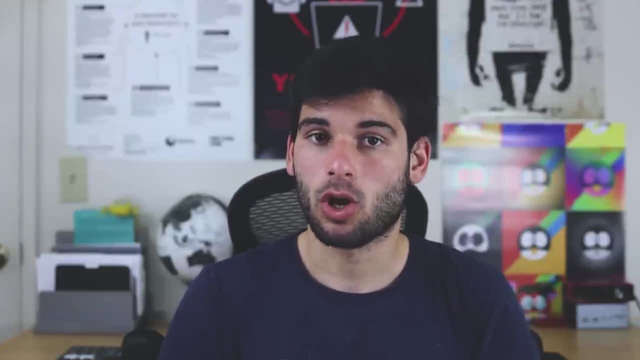 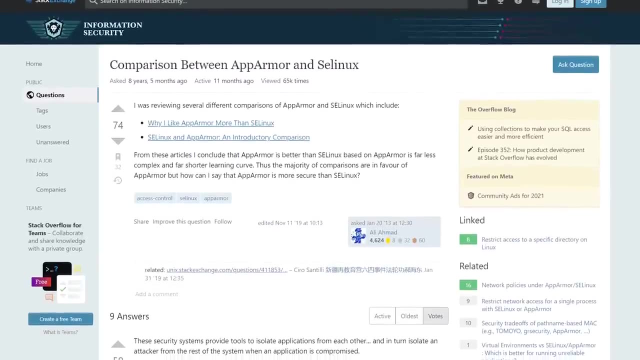 implies, it's an extremely valuable tool you can use. It is very much a more complex tool and there are active debates regarding SELinux vs App Armor, which is what we just talked about, with, honestly, no clear winner. There's pros and cons to both of them All. we recommend 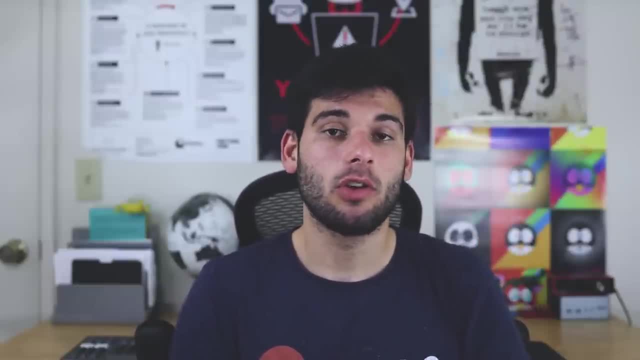 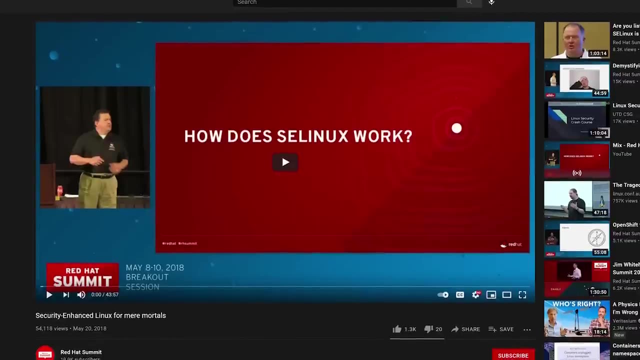 is you understand SELinux before deciding to use it or dismiss it. This video is a great introduction to SELinux and I hope you enjoy it If you want to learn more about SELinux, and we recommend everyone watches it after they're done watching this video to help decide. 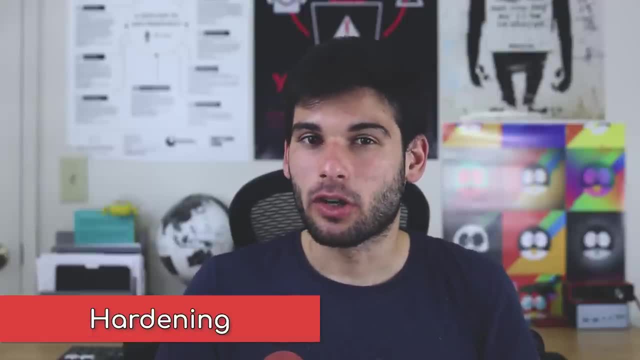 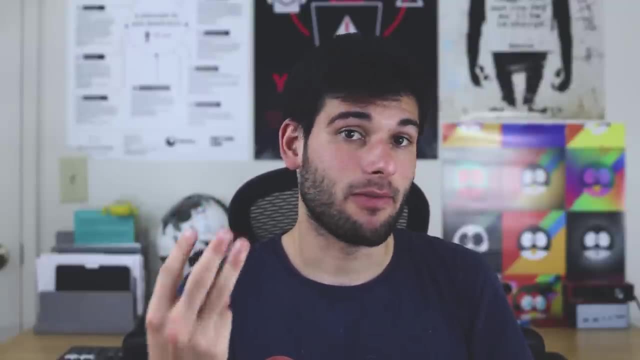 what's right for them. Hardening is simply a broad term for improving the privacy and security of Linux as much as we can. We've broken things down into Basic, Intermediate and Advanced. Links to all resources are down below. Basic mostly already covers things we've talked about. 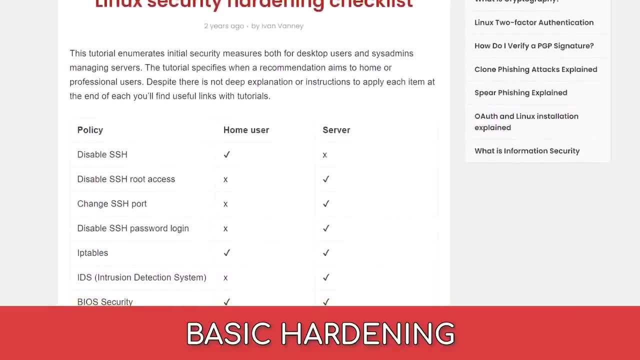 but it's still a valuable place to double check things and see if there's more you can do. Intermediate is from the Fedora docs, and we recommend diving through everything just to make sure you know what's right for you and what's wrong with you. 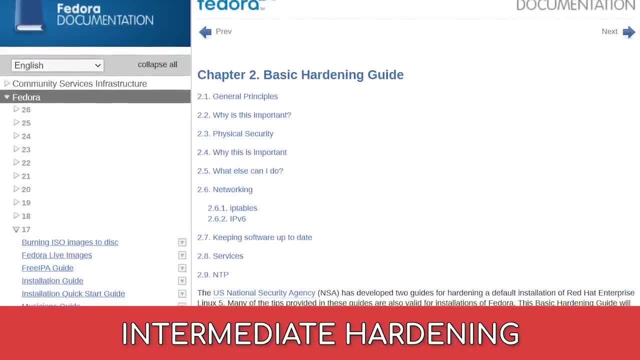 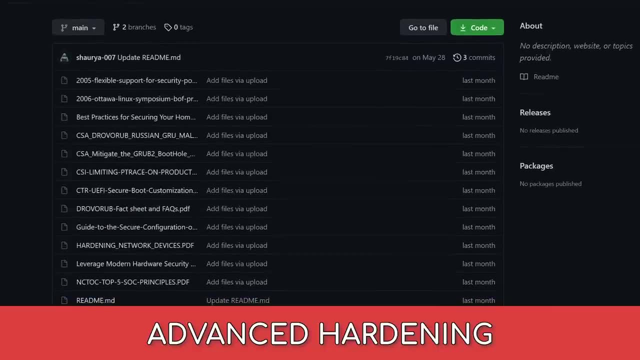 Just because it's from Fedora docs doesn't mean you can't apply this information to your chosen distro. Finally, we have someone who compiled a GitHub repo with tons of documents from the NSA, Linux hardening docs and some other great resources. If you want to spend a weekend reading through. 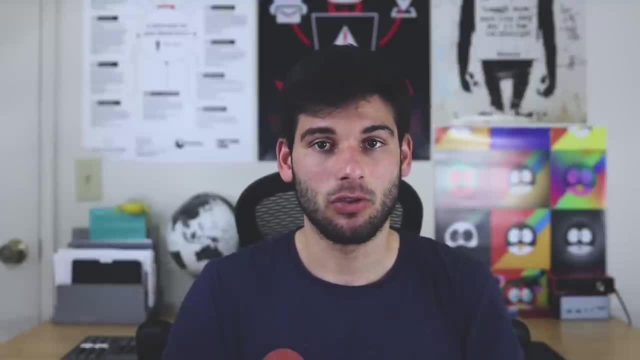 all of this and absorbing all of this great knowledge, that's the place to do it. Keep in mind that many of these more advanced hardening tips are well beyond the tipping point of diminishing returns and are likely for the very extreme threat models. and even then. 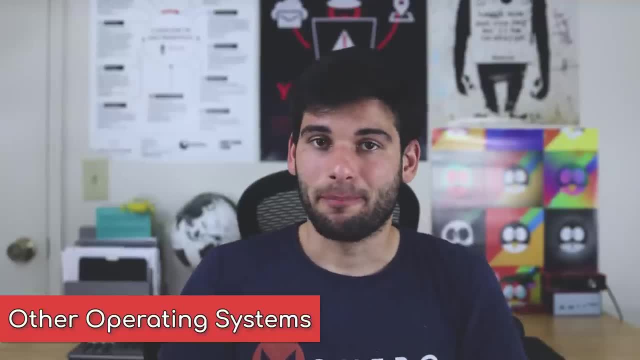 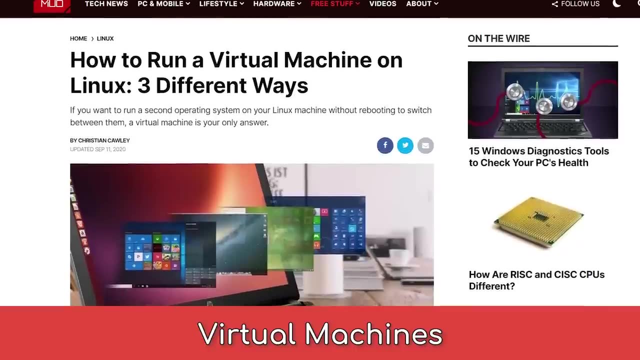 some of these recommendations are very much up for debate. We're almost done. Let's talk about other operating systems First, don't forget basic options like virtual machines, which are sandboxed operating systems running on top of your OS. You can have several virtual machines for different tasks to help. 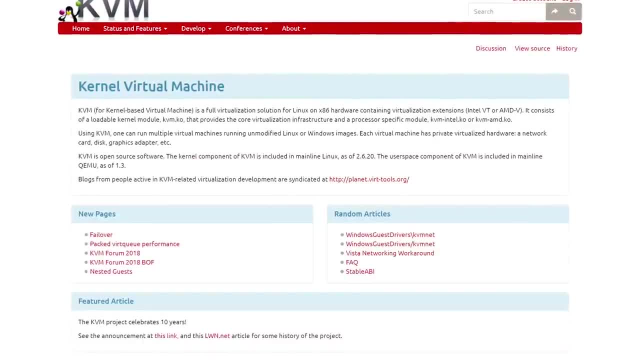 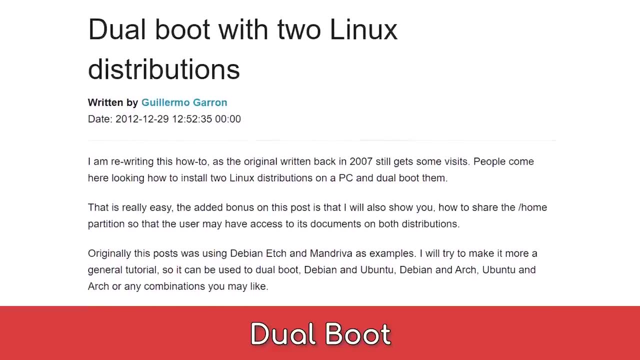 compartmentalize everything further. Also, you have KVM at your disposal, so really take advantage of that. Alternatively, you can dual boot different Linux distributions for different tasks if you find one distro is better for you than another in one given part. 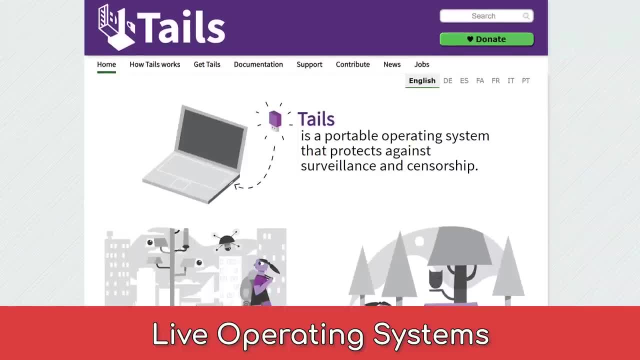 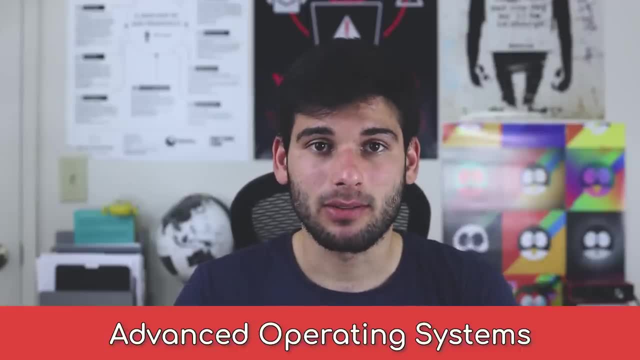 of your life. Don't forget: you can use live operating systems as well, like Tailgate or Tails OS, if you want a non-persistent location completely separate from your main operating system. Finally, let's not forget the more advanced operating systems. Hoonix is a great operating.